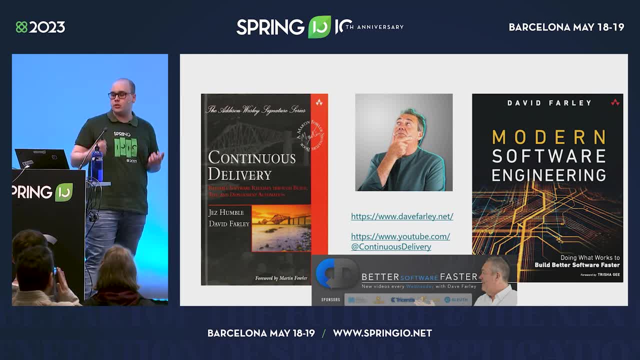 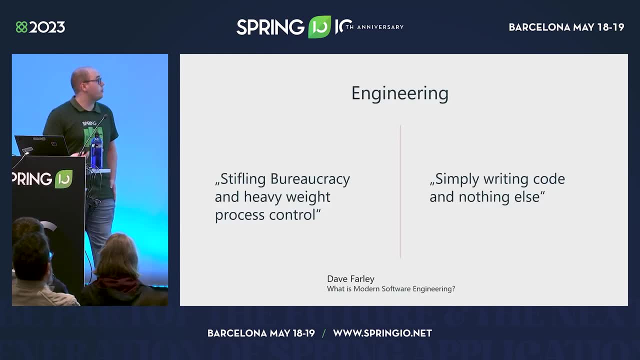 As a software developer, I always looked up to him as he shares his valuable insights and his real-world experience on his YouTube channel, Continuous Delivery. He shares his point of view on engineering in his blog post. What is Modern Software Engineering? He's uneasy with the term in the context of software development, as it is either incorrectly. 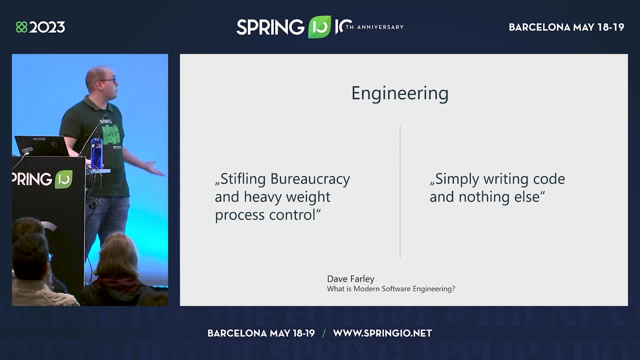 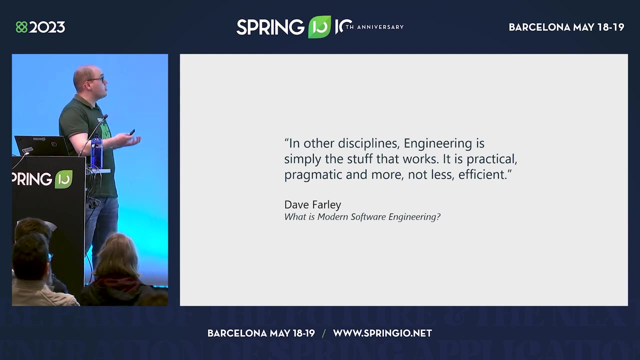 with meaning or emptied of it altogether. Some developers think it entails stifling bureaucracy and heavy white process control, while others think it's just simply writing code and nothing else. He tells us that both of these are profoundly wrong. In other disciplines, engineering is simply the stuff that works. 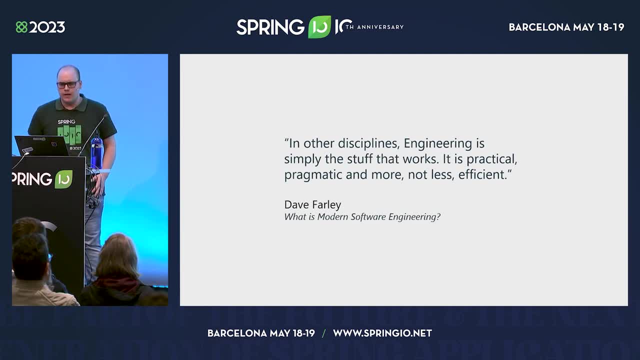 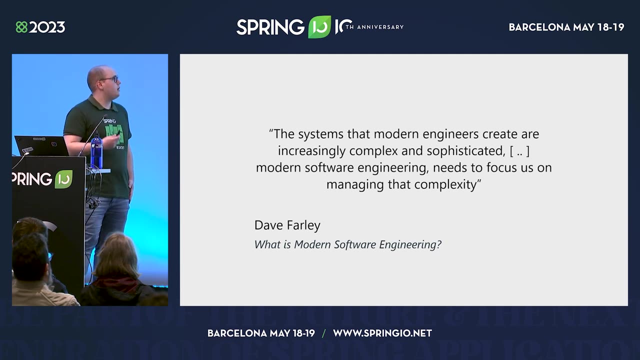 It's practical, pragmatic and more, not less, efficient. But is the way we build modern web applications practical, pragmatic and efficient? Could there not be a simpler approach that is sufficient for many use cases? today, The systems that modern engineers create are increasingly complex and sophisticated: Modern. 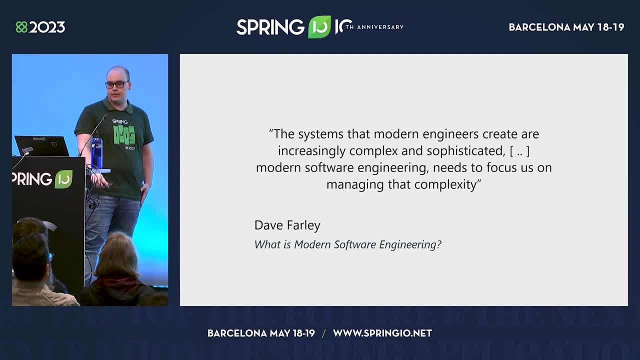 software engineering needs to focus us on managing that complexity. Farley concludes that if an engineering approach to software development doesn't help us to create better software faster, also It is wrong and it doesn't qualify as engineering. So did we overshoot this goal? 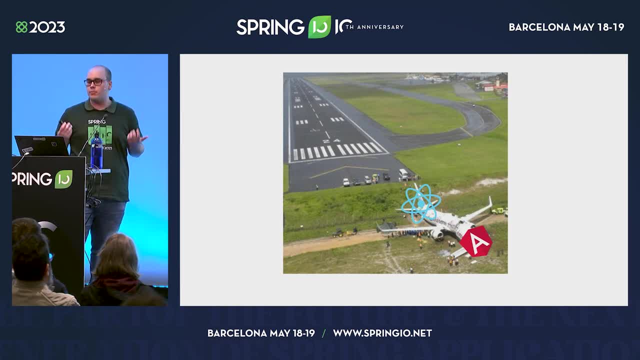 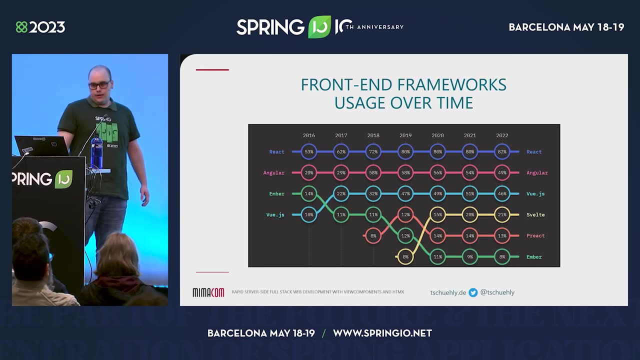 while trying to build more advanced systems than ever before to solve problems that we created ourselves? What if, instead, we tried to reduce complexity for our modern web applications that are not inherent in the challenges of our business, but accidental due to the nature of our solutions? Modern JavaScript frameworks were developed to manage the complexity of 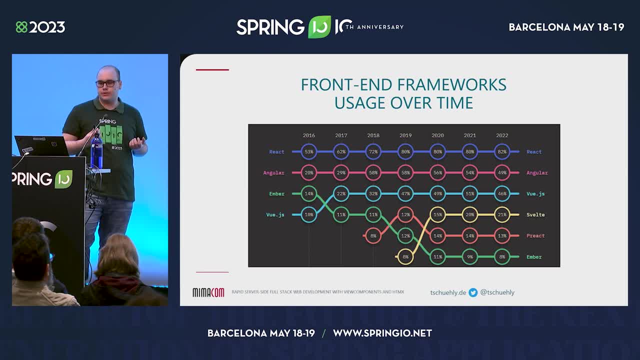 front-end development and improve the user and developer experience. They are mostly single-page applications, meaning a blank HTML and a big block of JavaScript gets delivered to the client to render the page on the browser. The most used JavaScript framework is React, with 82 per cent of developers who answered the state of JS survey 2020 used it. It has 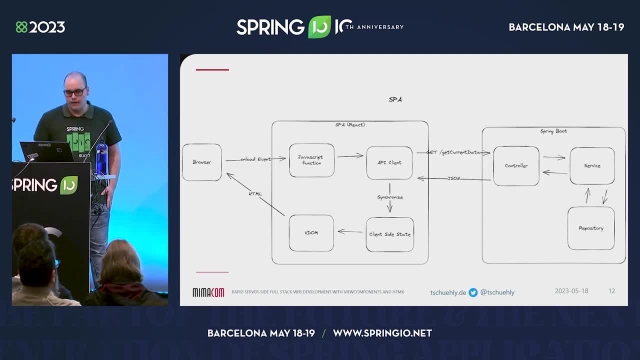 grown to the de facto norm for building web front-ends. Here you can see what a typical single-page application looks like. It is a single-page application with a single-page application render process. The browser calls the JavaScript function. This function again calls an API client that fetches the data from our beautiful Spring Boot back-end. 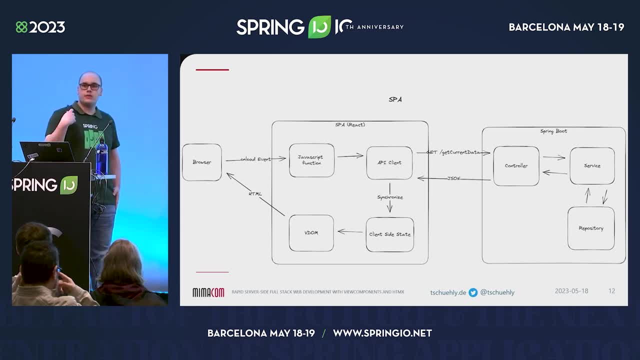 The back-end fetches the data from our database and then has to transform it into a POJO. The POJO then gets serialised into Jackson. The API client then has to deserialise the JSON into a JavaScript object. The single-page application then needs to merge these changes. 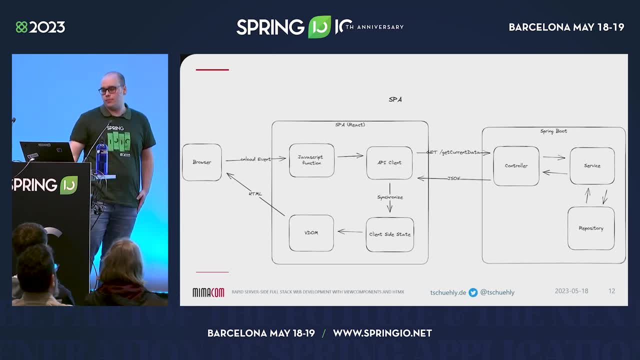 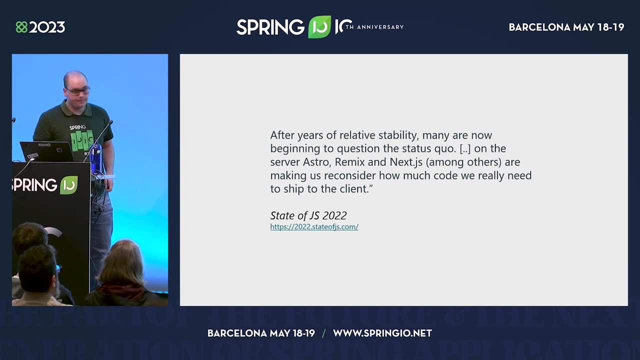 into a virtual one. The single-page application then needs to merge these changes into a virtual DOM and the virtual DOM is synchronised with the actual HTML browser DOM. The JavaScript community started to question the way most modern web applications were built over the last decade. In the intro to the state of JS survey reads: after years. 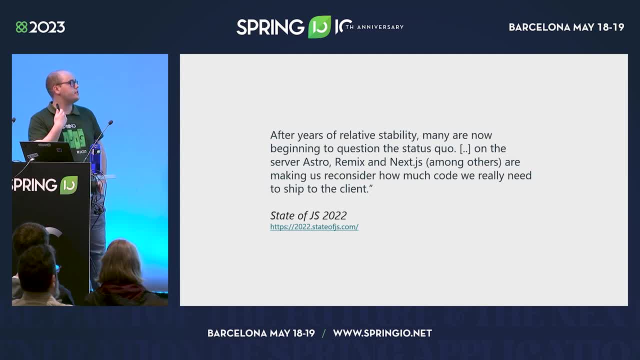 of relative stability. many are now beginning to question the status quo On the server. Astro Remix and Nextjs, among others, are making us re-concentrate on the fact that we need to re-consider how much code we really need to ship to the client. But even if the 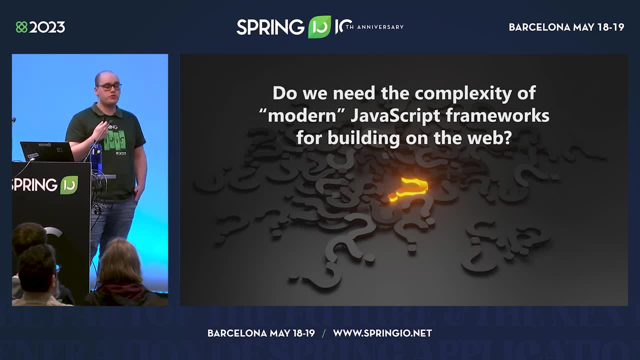 JavaScript fanboys tell us that we shouldn't ship much code to the client. why do we need this complexity? The JavaScript frameworks come out of the box. There are certainly use cases where we need sub-millisecond responses on a dynamic UI, but does anyone think all? 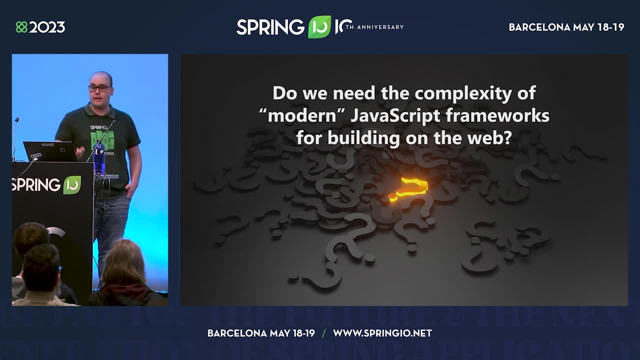 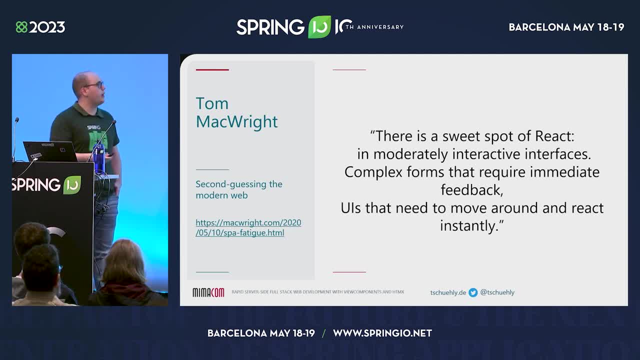 Tom McWright puts it nicely in his blog post. Tom McWright puts it nicely in his blog post: There's a sweet spot in Re-Act: in interactive interfaces, forms that require immediate feedback and UIs that need to move around instantly. I agree that there are many applications that 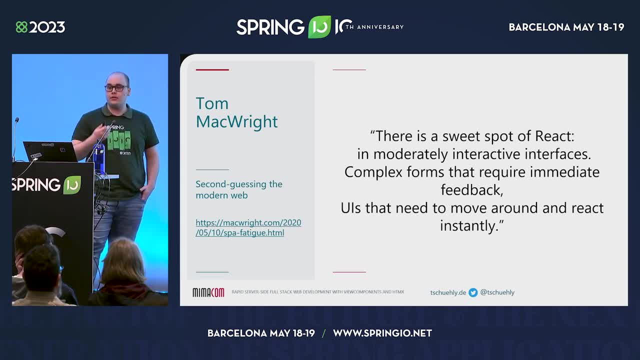 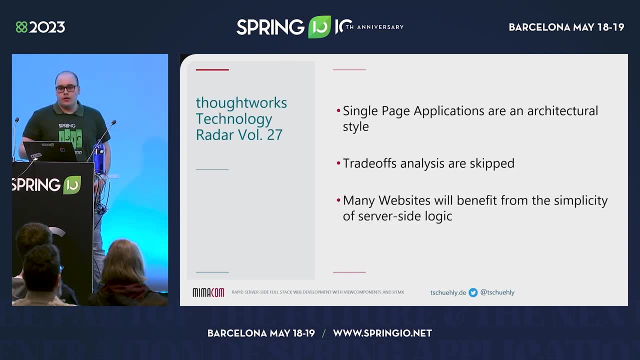 need this kind of user experience, But I think even more apps don't need this level of extra interactivity or could benefit from a simpler approach. The excellent engineers that contributed the Thoughtworks technology agree: single-page applications are an architecture in itself. Nadia analysis, Please baptise the proof of. 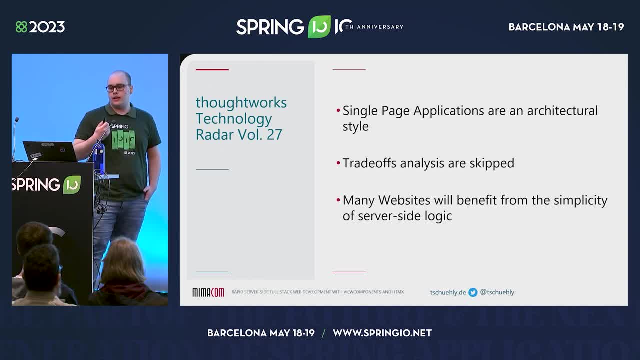 – Ok, thanks, style that should be chosen after proper trade-off analysis and like the additional complexity a single page application implies. The problem is that nowadays this analysis is often skipped and is not evaluated. if the requirements even need a framework like React, Many developers nowadays are not even aware. 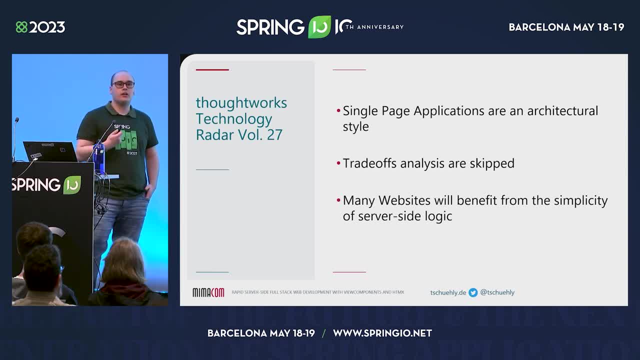 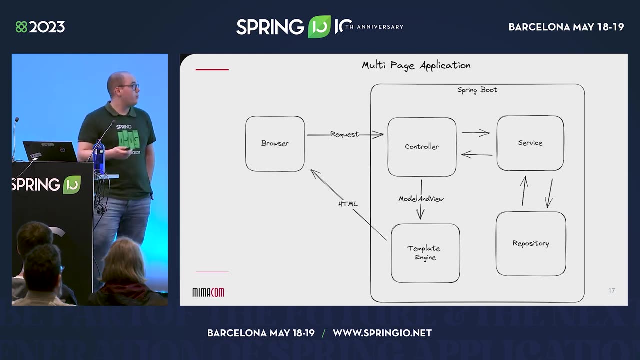 that other possibilities exist, because they spent their entire career in a framework like React. The ThoughtWorks technology radar concludes that many websites will benefit from the simplicity of server-side logic. Most of you that were developers before 2015 probably built web applications with the. 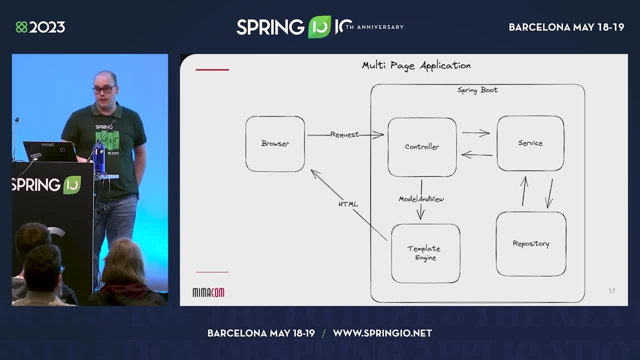 traditional approach to the web multi-page applications. The approach is quite simple and still powers most of the web today. Instead of shipping a blank HTML and a giant JavaScript bundle to render the pages on the client, we just ship the HTML the browser can display directly to the client and 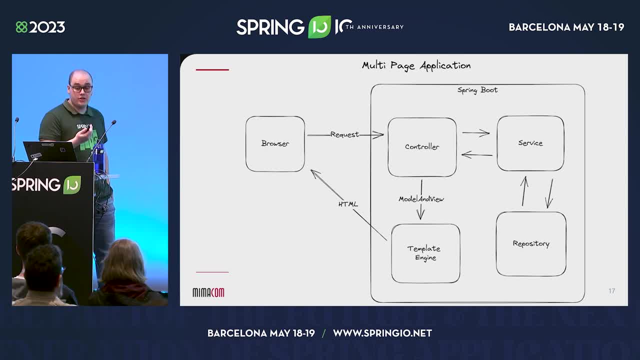 having no over-the-top functionality, Spring can serve HTML to the browser directly. When a request goes to a controller. the controller then fetches the data from our database into a model. The HTML template that we create is the view, and these both are. 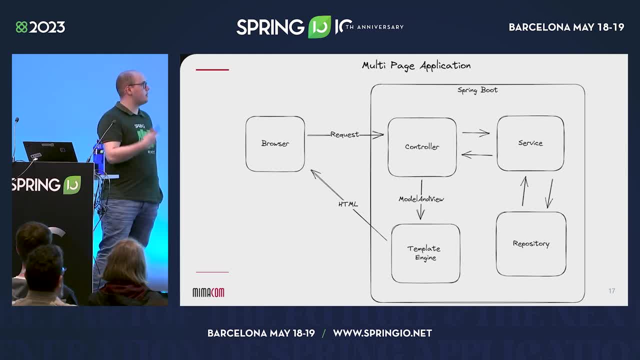 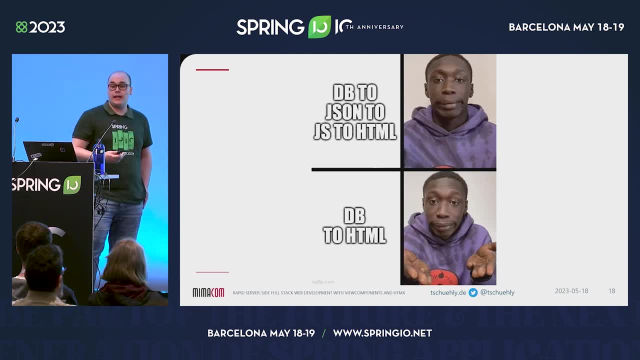 passed into the template engine as model and view. that renders our HTML and returns it to the browser. Sounds awesome, right? We removed a whole lot of complexity by removing two data representation layers between our client and our data. We lost some interactivity, though, because we just shipped static HTML without any client-side JavaScript, So how? 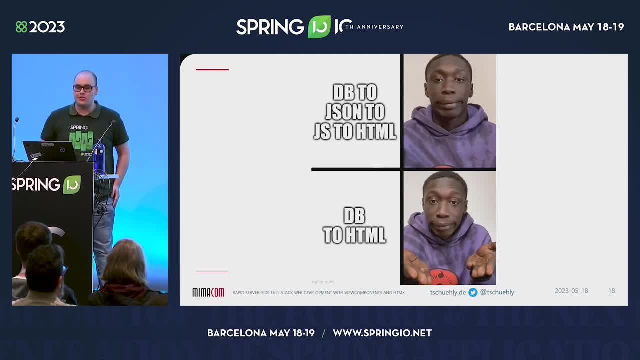 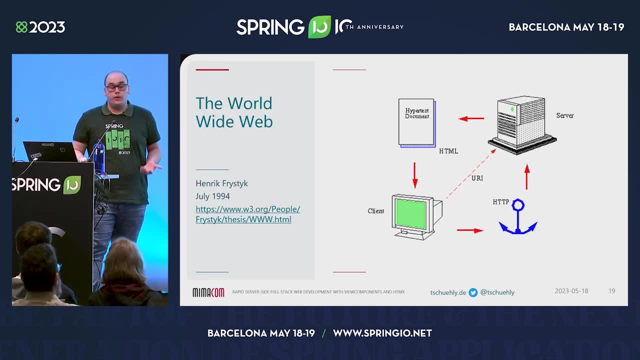 can we return the JavaScript, the interactivity, to our server-side rendered web pages? To solve this question, we need to look at the original model of the World Wide Web and focus on the hypermedia essential to even the most over-engineered JavaScript pages. 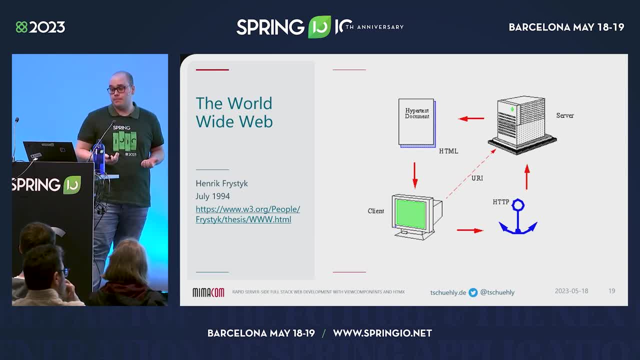 Because in the end, the browser can only display the hypertext markup language. So why not redevelop it over the HTML of the hypertext transfer protocol, like Tim Berners-Lee did in 1989, when he invented the World Wide Web? Hypertext is a form of hypermedia. Ask. 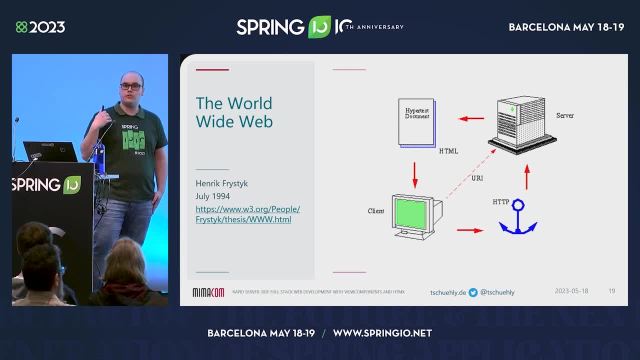 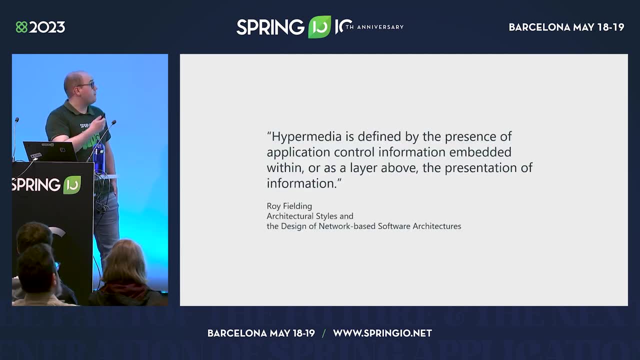 your younger colleagues if they ever heard of hypermedia. Not many tutorials nowadays cover the fundamental platform of the World Wide Web. Hypermedia is defined by the presence of application control information. What does fielding want to tell us, with this quite academic definition, When we deliver? 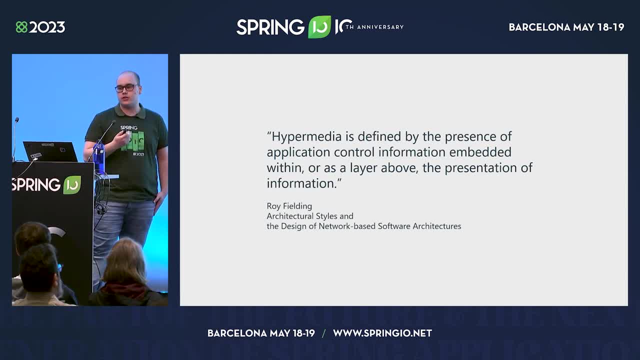 hypermedia to our clients. we also deliver the possible interactions the client can do. The most common control, you probably all know, is the anchor tag or hyperlink. It enables us to discover whole applications without any documentation. Or when was the last time you had to read documentation to order cat doors from Amazon? 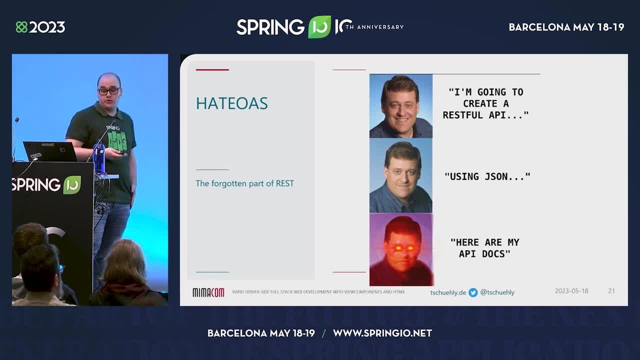 Hypermedia as the engine of application state is a constraint of the REST application architecture that distinguishes it from other application architectures. With Hadeas, a client interacts with a network application whose application servers provide information dynamically through hypermedia. The REST client needs no prior knowledge of how to interact with the server. 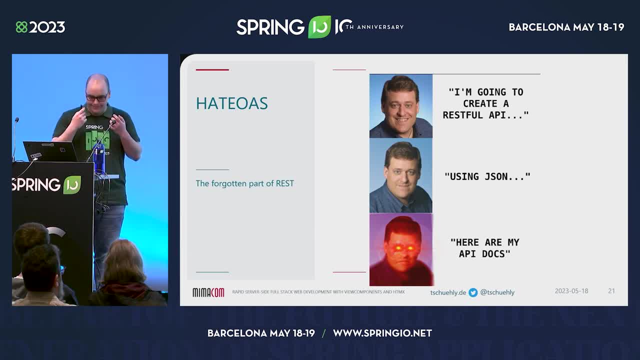 besides a general, a generic understanding of hypermedia, HeyDios decouples the client and the server at a network level and enables us to evolve them independently. Ask yourself: do you need a lot of communication between your front and your backend for API docs if you want to evolve your single-pager application? 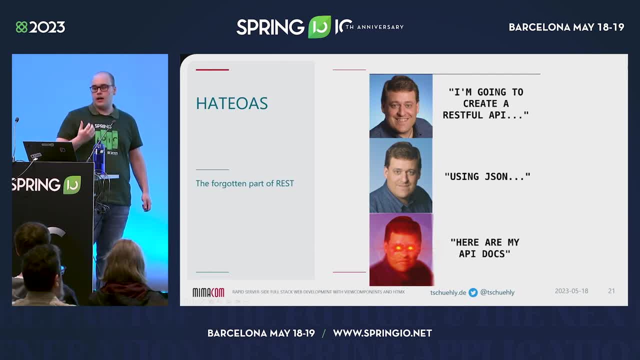 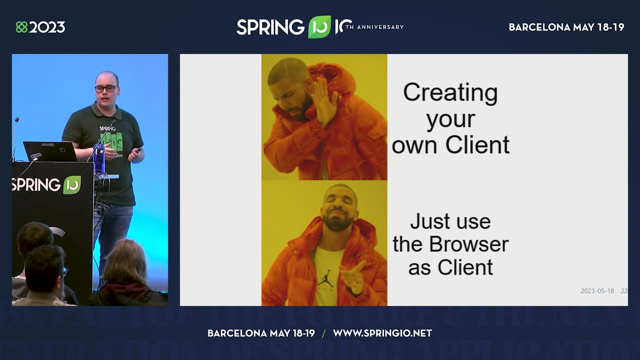 The JavaScript frontend need intricate knowledge of your backend API, because they need the correct information and structure to render the HTML correctly. So why decouple at an application level between the template and our data with JSON? Another interesting fact of HeyDios is that we don't need different roles for the client. 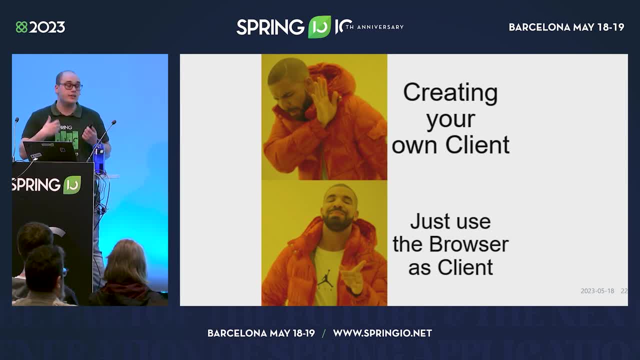 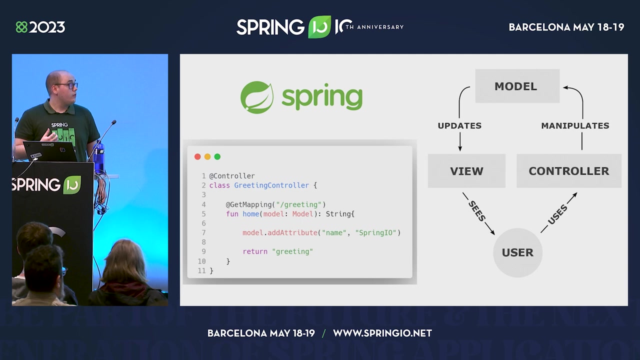 and the server, because we don't need to develop our own client. We just use the hypermedia client, available to all our users without download, built by some of the smartest engineers at Google. Thank you, We reduced the complexity. We can fill HTML with data from our database when we deliver it to our user with Spring. 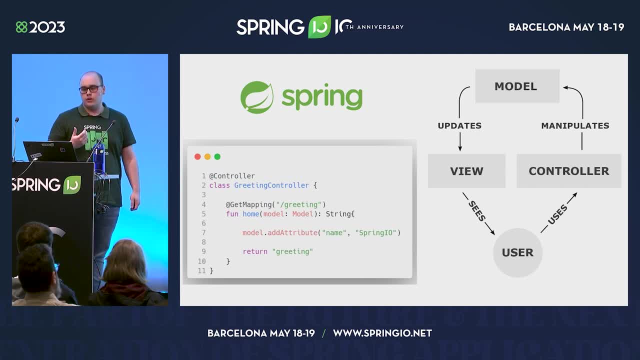 as well. Spring uses the ModellView controller pattern to server-side render applications With MVC the controller view developer to save dataset package, say. vendor 그래요 is responsible to receive the request. Here you can see a get mapping with a path greeting. 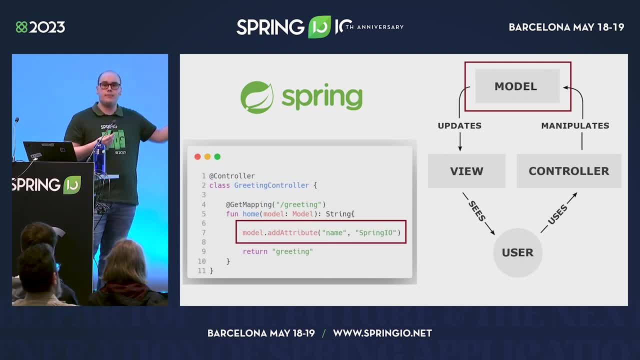 The controller then changes our model. Here we add the attribute name Spring IO to our model. Then we return the name of the template we want to render. Here it's a greetinghtml that lives in our resources folder. There are multiple template engines to render dynamic. 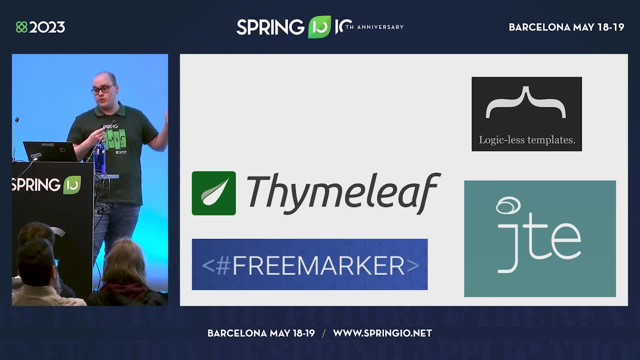 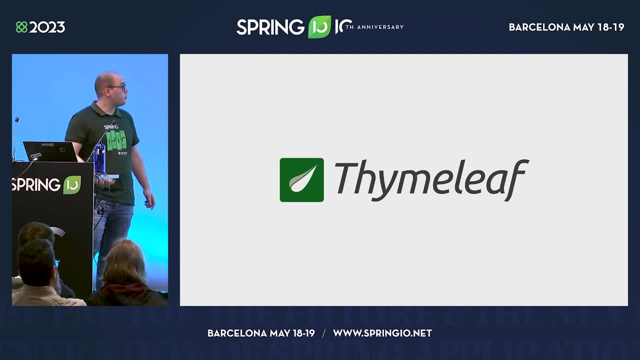 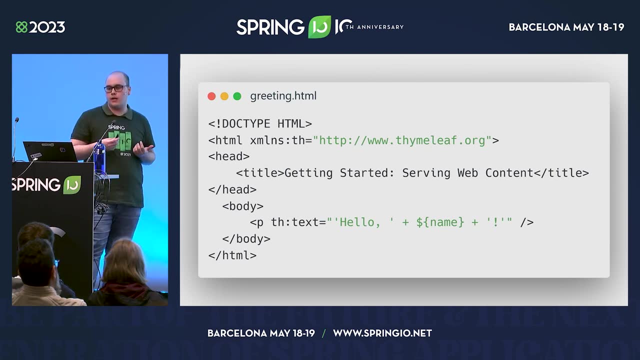 data with Spring, like Apache, free marker and. but today I will look at time leaf and JTE, the Java template engine. First we will take a quick look at time leaf. It is quite simple to render some crispy HTML. This is the greetinghtml we just returned. 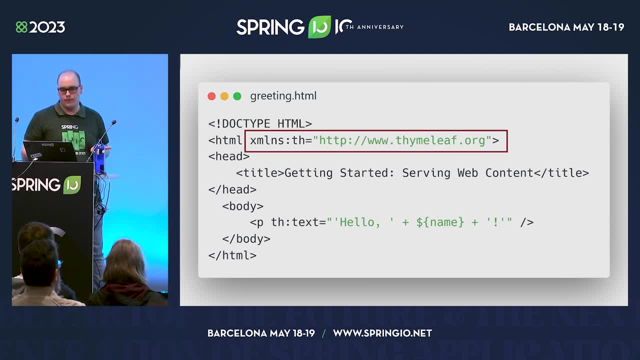 from the browser. It's just boxed in our HTML. We added a little tag at the top, so is picks up the template language To render our project. we next click on a clickhtml order. We do that in a different our data. we use TH attributes. Here it's the TH text attribute. It has hello spring. 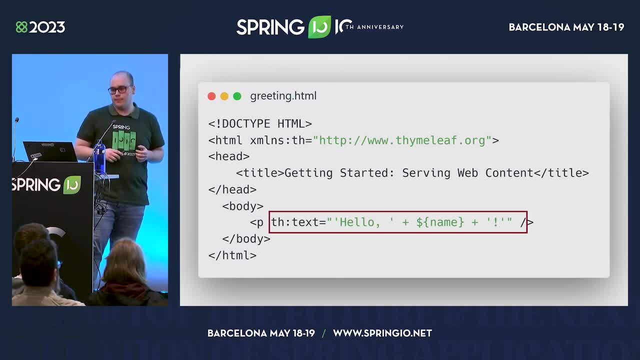 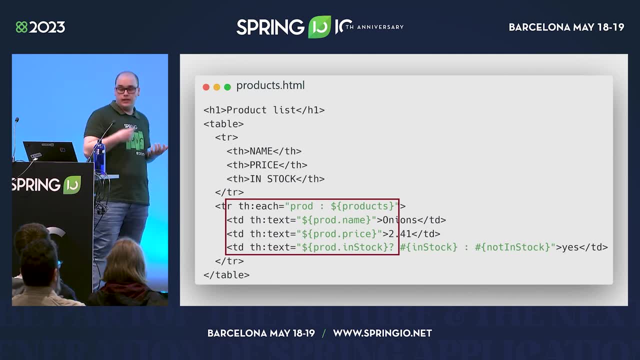 IO to the inner HTML of our P tag The name. we use the name variable from our model. We can also do stuff like iteration over list. Here we iterate with the TH, each attribute over the list of products. Then we show a table data cell for each property of the object. 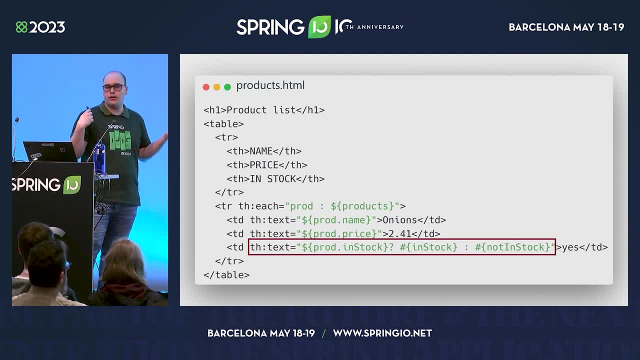 Examples are also very simple. We can use the ternary operator. you might know from other languages. If the in-stock evaluates to true, we show the message not in stock. The message in-stock. If it is false, we render the message not in stock. There are even more features. 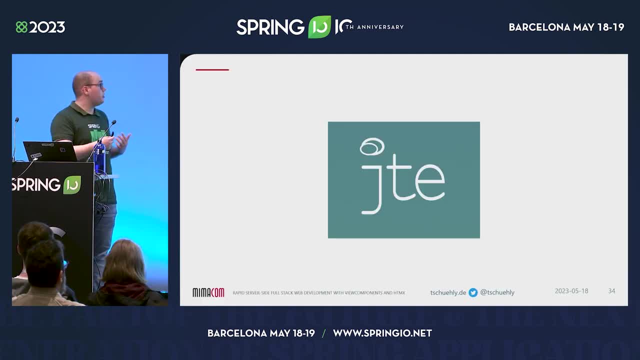 but I will not go more in depth in this talk. Next we will look at the JTE, the Java template engine. It might feel more natural to Java developers and it has an awesome plug-in that makes it easy to use. It's also very easy to use. It's also very simple. We can. 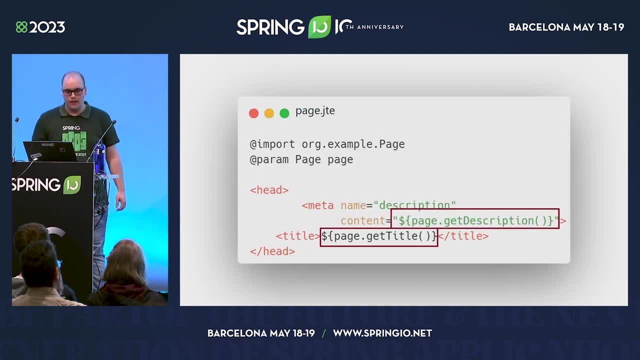 use plain Java expressions right inside our HTML with a dollar sign and curly braces. We can either use them inside attributes or inside our HTML directly. JTE templates are compiled to native Java classes. To import the classes we use, we use the syntax. We also need to declare the. 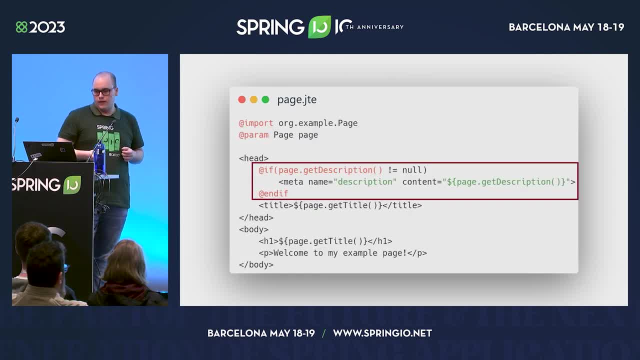 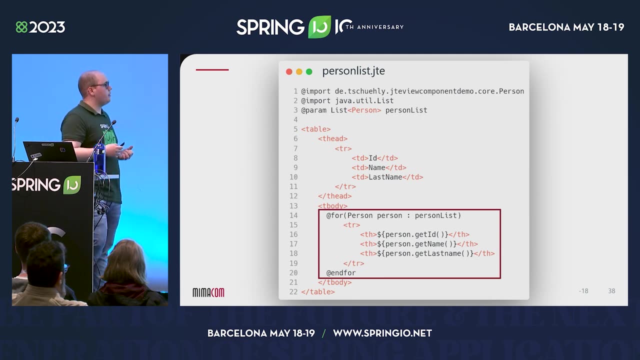 list, in our model with the add perm annotation. We can also use control structures like ifs. Here we check if the page description is unequal null and then show the meta tag. We can also do for loops with JTE. Here we loop over the list of persons and then show a table. 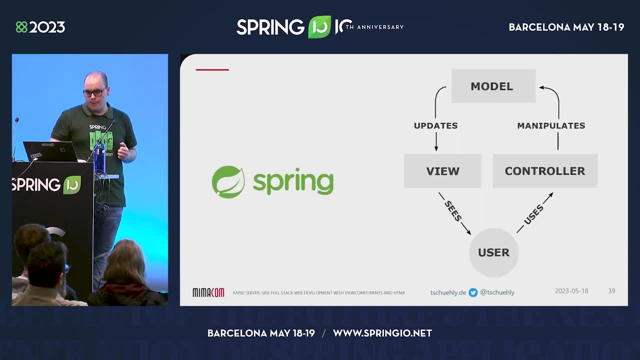 header for each person and property. MVC is quite simple, but it has some shortcomings that bothered me while I was building my software as a service side business. over the last year, The two most popular JavaScript frameworks were built by some of the smartest software engineers at Google and Facebook, and they 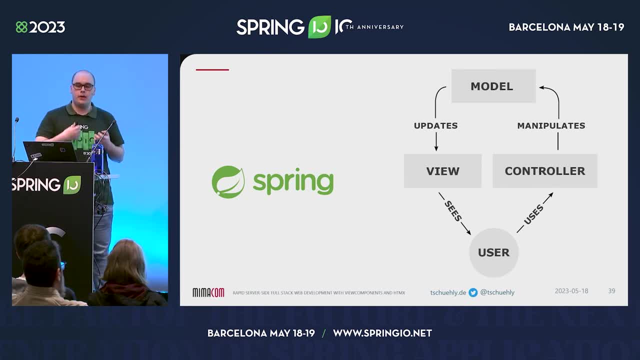 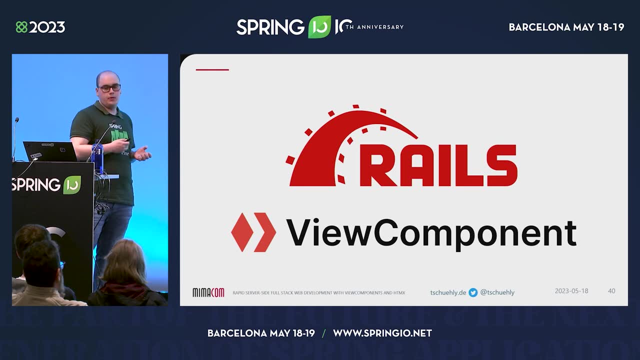 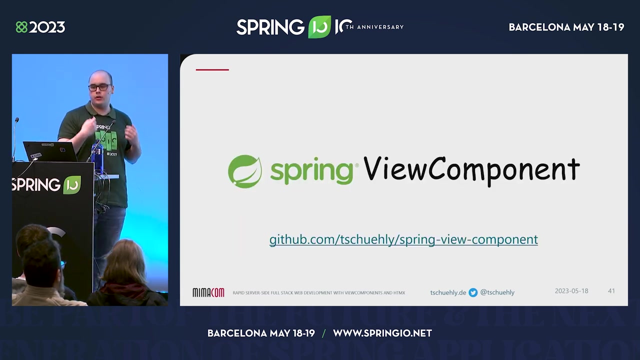 built their UI based on components, because components make the UI reusable and structured Components are so cool that even GitHub built their own view component library for the Ruby on Rails server-rendered parts of GitHubcom. but they ran components to create a reusable, type-safe UI with Spring. But fret not, I've solved that with the Spring view component library. 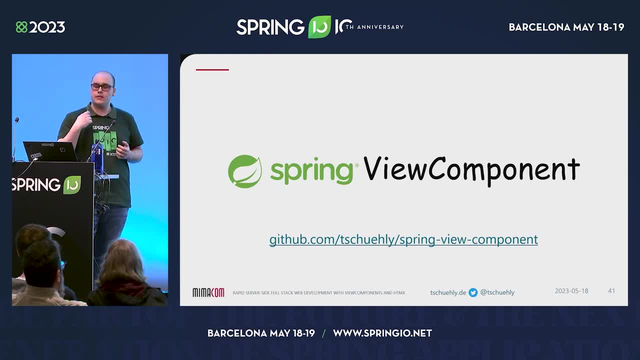 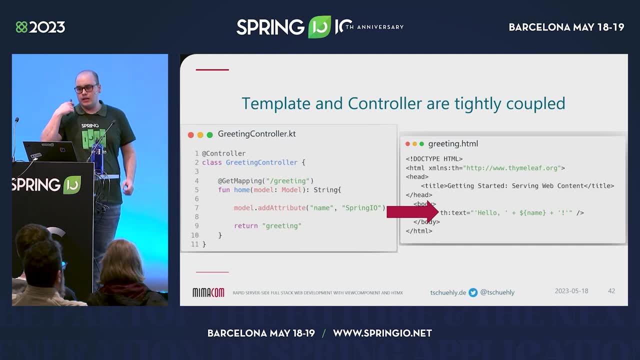 I can show you how we solve the issues that occur with an MVC approach. The first problem with MVC is that our controller has to have intricate knowledge of what variables we need in our template, tightly coupling your controller to our view. There are no compile-time checks if the model properties are even available, This gets. 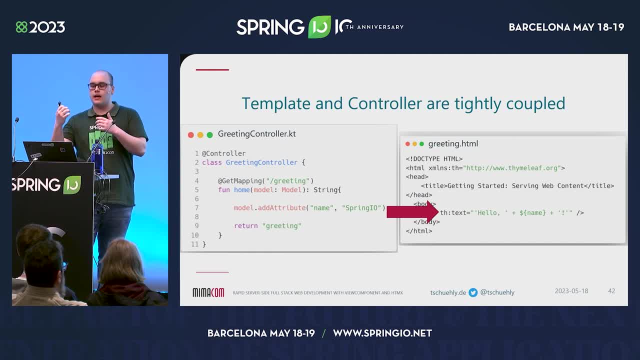 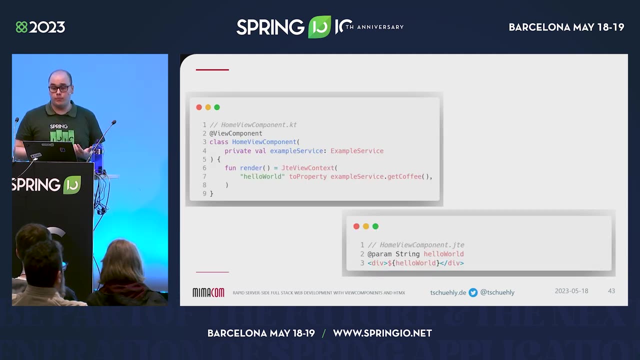 especially spicy if we reuse templates inside other templates. For example, if we change a variable we need to change it in every template, in every model that the controller method returns that template. To solve this we use Spring view component. We can create: 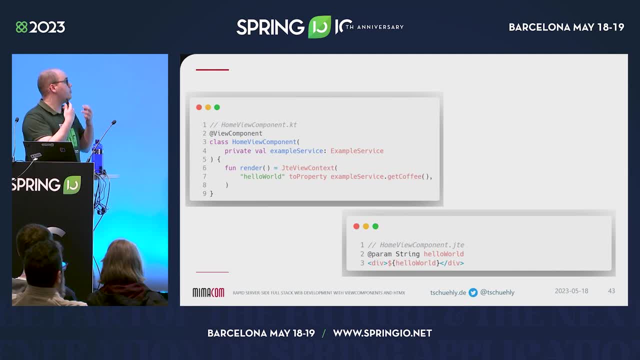 a component with the add view component annotation, making it a Spring-managed bean, enabling us to dependency-inject services, for example. We then define a random method that returns a view context. Here we use the JTE-specific JTE view context. We create a hello world. 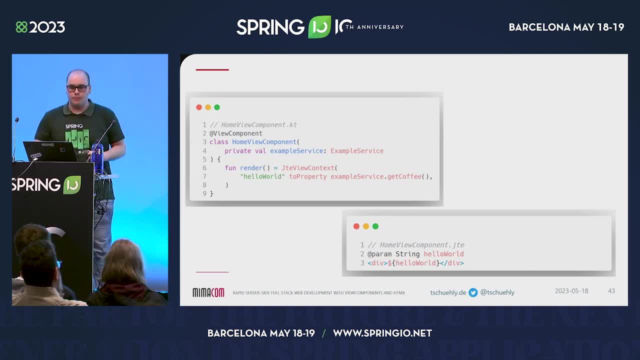 property and get the data from our example service, making it available to our template. Then on the bottom left you can see the template. It needs to have the same name as the component in the same package Inside our template. we can then. 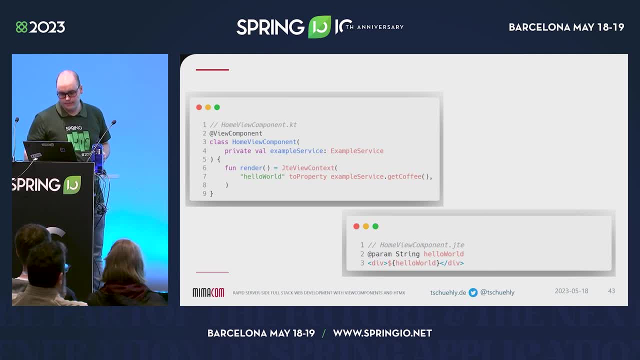 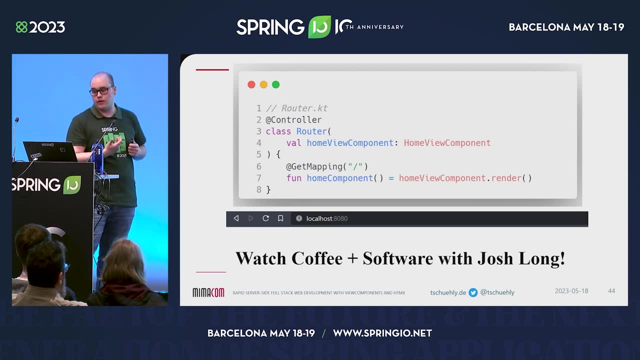 use the properties we defined in our view context To display components. when we want to navigate to a certain route, we call the HomeViewComponentrandom method and return it in our controller method. We now have a clear separation of concerns- The controller. 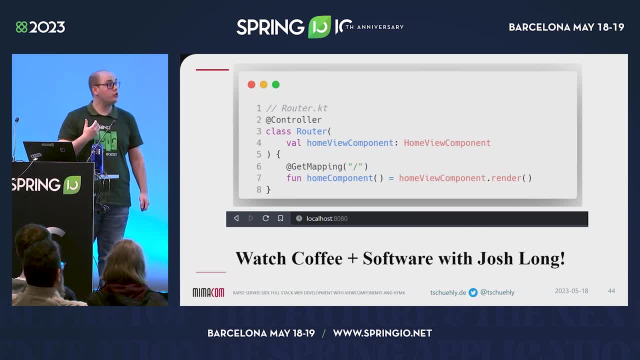 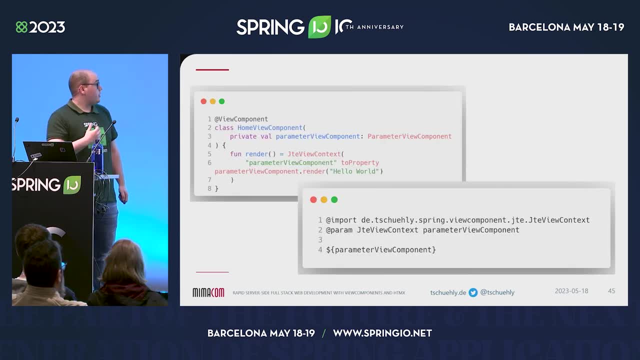 is responsible for routing and not for data fetching, and the view component is responsible that all data is available at the time of render. We can also nest components to make them reusable. Here we pass the view context that the parameter view componentrandom method. 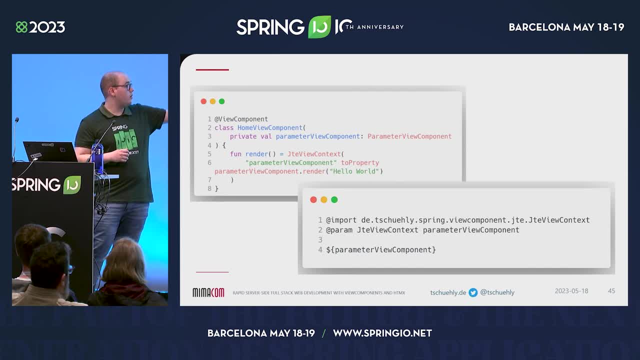 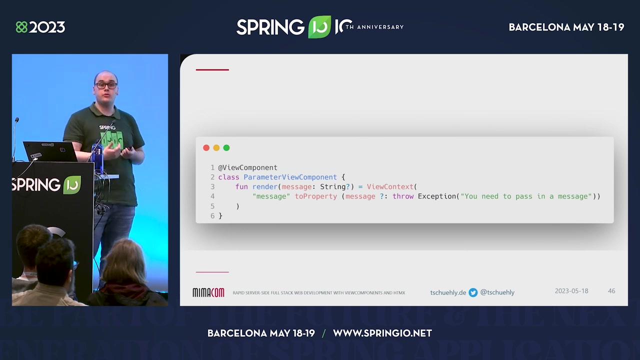 creates to our template, Then inside our template we use the JTE view context inside a JTE expression. The HomeViewComponent is an independent component as it fetches the data itself but making it less reusable. The other type of component is the parameterized view component. It does not do any data fetching. 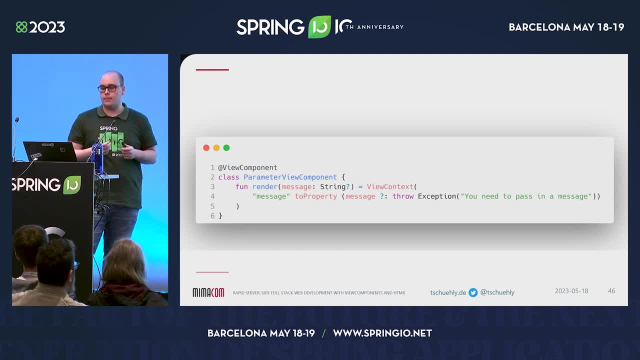 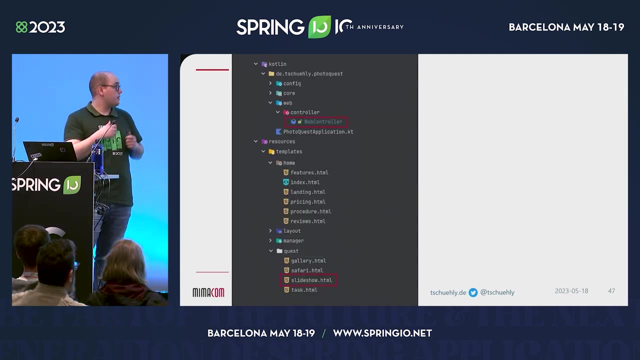 but instead relies on the parent component to pass the data. We can reuse these components everywhere in our app and give us the ability to create type-safe templates for commonly used UI patterns. Another problem with MVC is that the templates need to live in a resources. 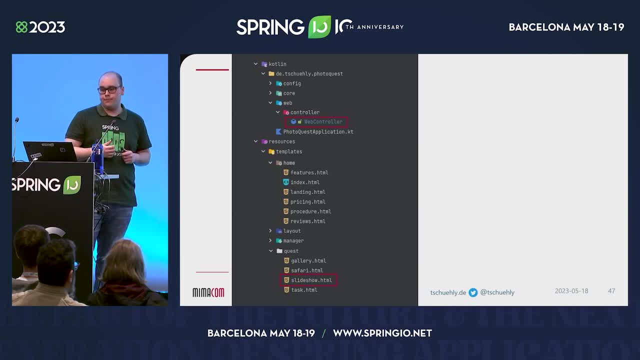 directory. While our control system is not able to do that, we can use the JTE view context to create them. The controller lives in the Kotlin directory. We have a strong disconnect where we aggregate our data and where we use it, thus having a low cohesion, which adds cognitive load when 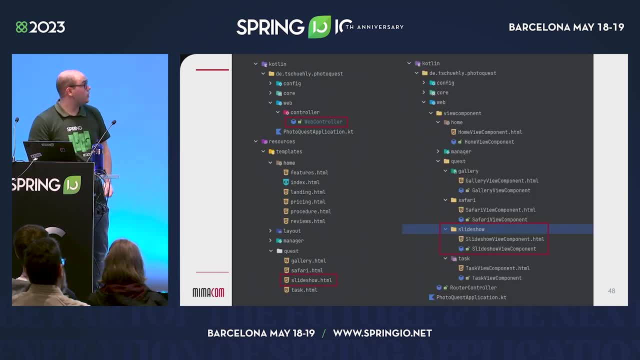 we try to evolve our front-end. With SpringViewComponent we can have a highly cohesive code structure, as the template needs to live in the same package as the data provider. It enables us to create completely feature-based package structures With MVC. on the left you can see that our slideshow features a 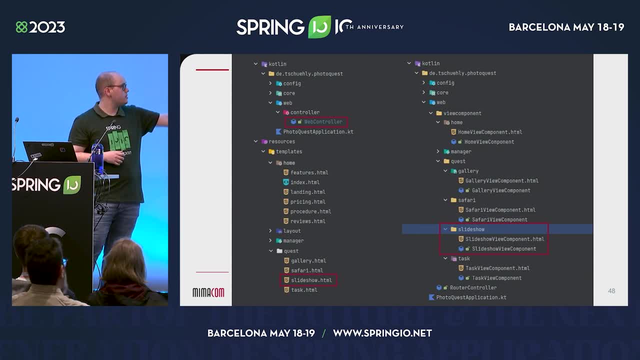 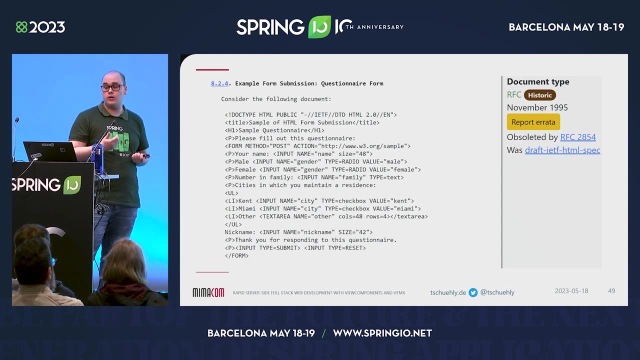 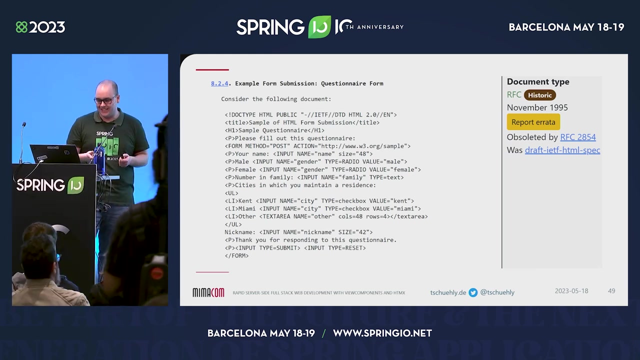 split in the resources directory and in the web controller package With ViewComponent. it is nicely packaged together in a bundle, in a slideshow bundle. So why did we move away from the hypermedia model to the JavaScript dystopia we have today, if it is so simple to create HTML on a client, on a server? Because we did? because HTML did. 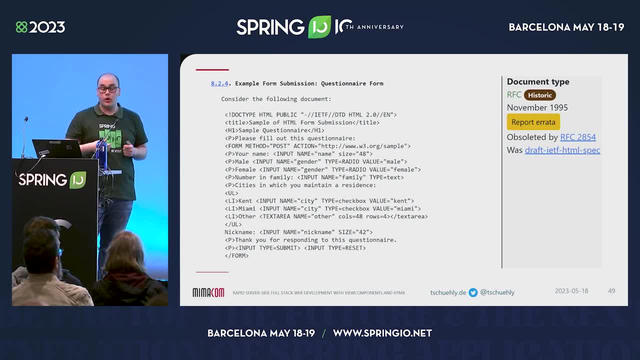 not evolve HTML evolved as a hypermedia. We only have two hypermedia controls: the anchor tag. that enabled the fundamental model of the World Wide Web. The World Wide Web is a hypermedia system that interconnects resources through your eyes. The second element is the form. 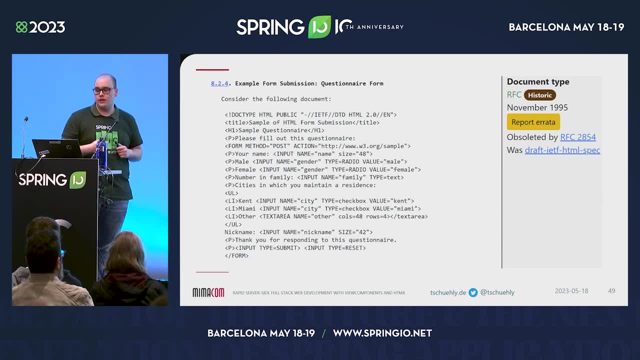 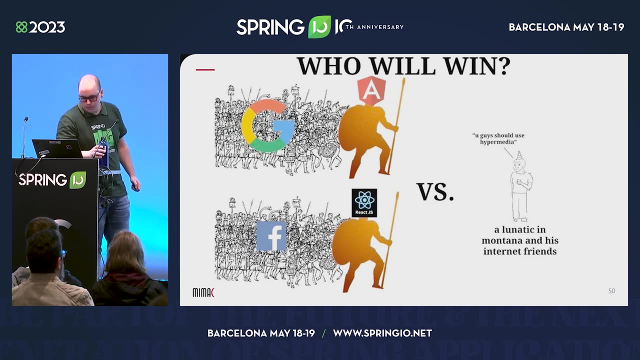 element. It was introduced in the HTML2RFC in 1995.. It made transactions for the first time possible in this vast hypermedia system. But it is still the same as it was 28 years ago. But one guy in Montana and his internet friends were not satisfied with that and created a. 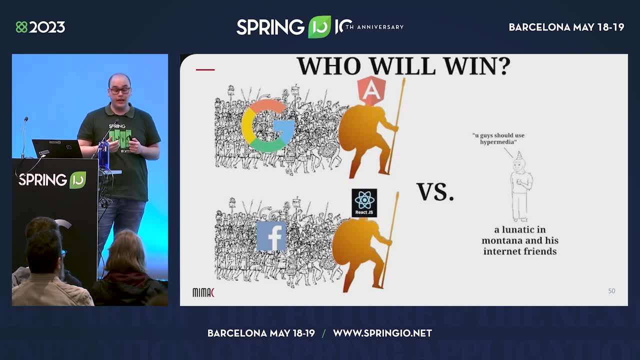 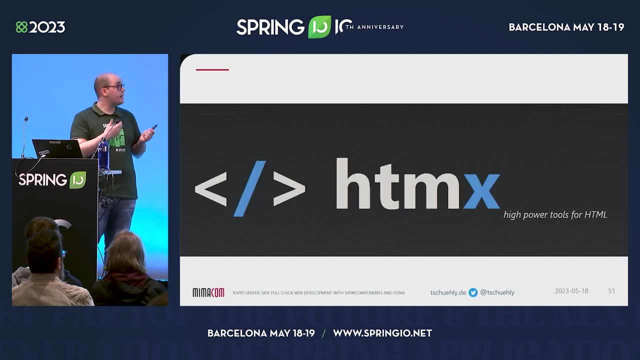 library to complete HTML as a hypermedia and compete against the giant JavaScript ecosystem fueled by big tech as we know it today. This library is called HTMLX and it has gained quite a bit of attention over the last year. GitHub recently picked it up in their original. 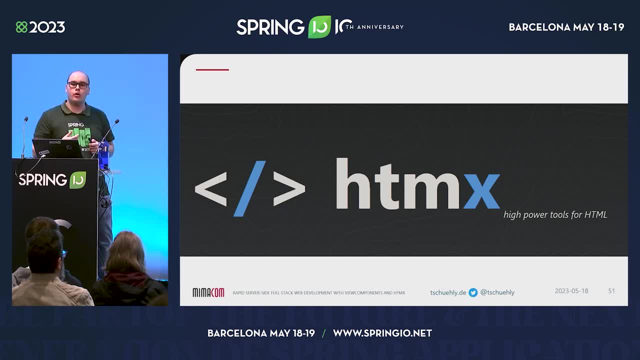 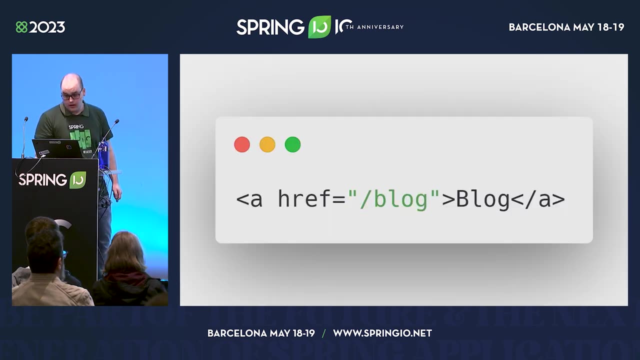 open-source Accelerate program. In a nutshell, HTMLX enables us to use modern browser features without ever leaving our HTML. it makes features interactive without ever needing to touch any JavaScript. To understand HTMLX, we first look at the anchor element. I think our element, the anchor- 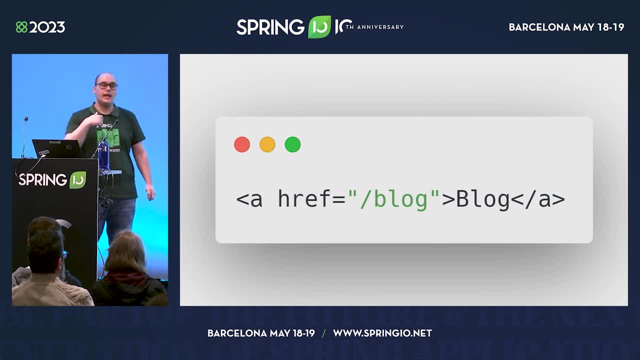 element tells the browser that when the user clicks on it, that it makes an HTTP GET request to the Control. Canvas港見 Z? louder săearä Goneоваä Ä? v13 Mobile Plan: Development ministers has the right to look at the energy engine. enfant personasä Är gehört. First choice in the event 술 ab. 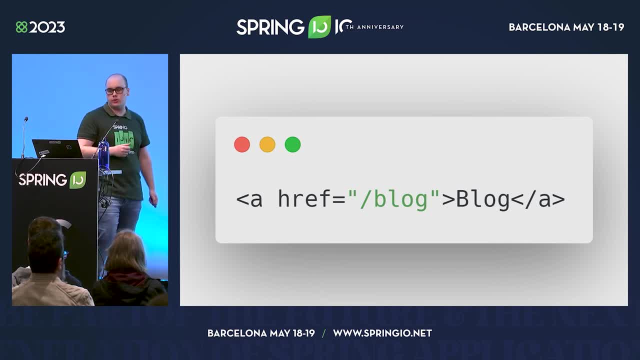 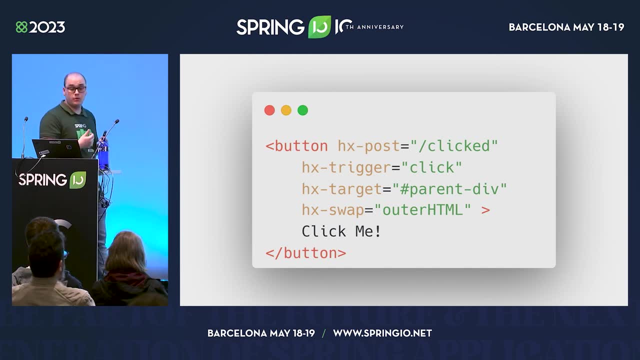 end point. We then load the response into the HTML browser window. Here is a simple example of HMX. It issues a post request to the slash click end point and then, when the content is loaded into, and then the content of the response is loaded into the ID with: 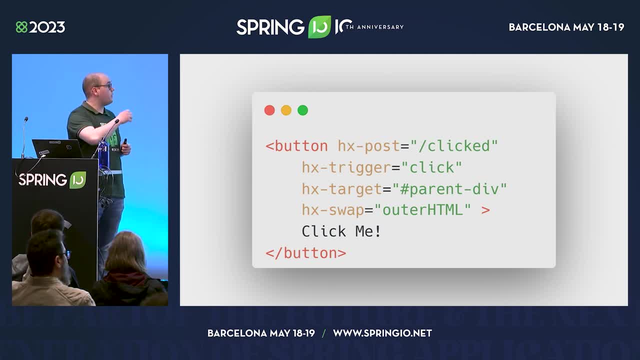 the parent div with the HX target attribute. We then swap the outer HTML. so we swap the whole element. HMX has sensible defaults Here. the HX trigger attribute is not needed as it is the standard behavior for a button element. HMX extends and generalizes the core. 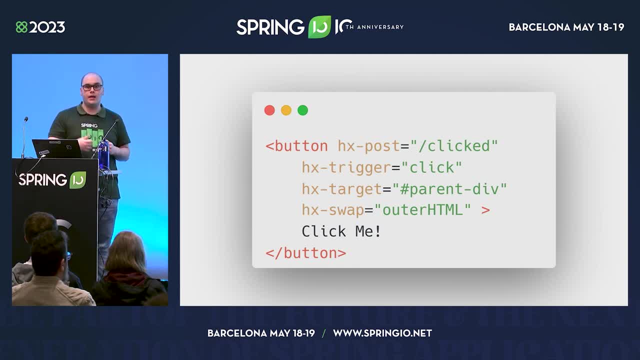 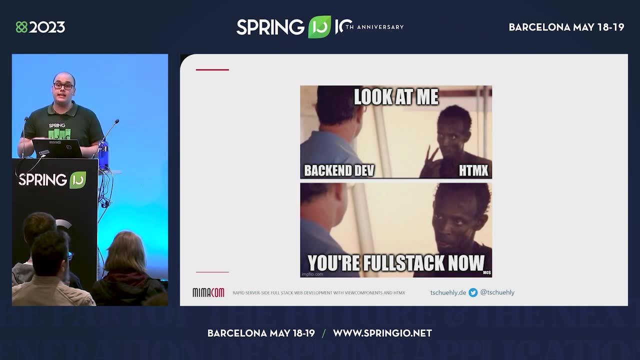 ID of the HTML as a hypertext and adds many more possibilities directly within the language. We enable developers to easily create full stack applications because any element can create HTTP requests. Now any event, not just click and form submission, can trigger requests. Now any HTTP verb, not just get and post, can be used. And now any element, not just 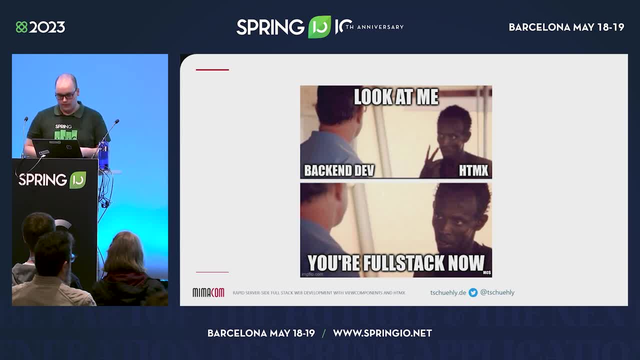 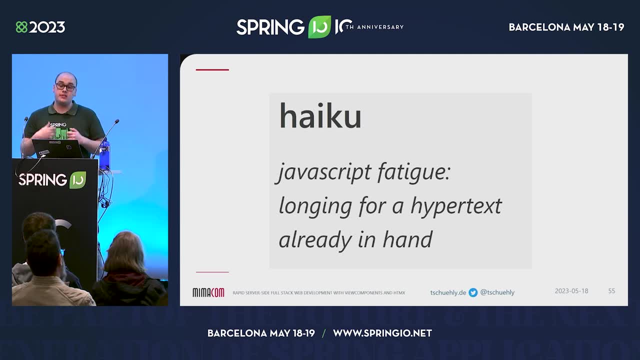 the entire window can be targeted for updates. HTMX refers to this style of application as a hypermedia-driven application, or HDA. It tries to capture the advantages of both multi-page application and the simplicity and flexibility of it, with a restful application architecture and happy media as the engine of application. 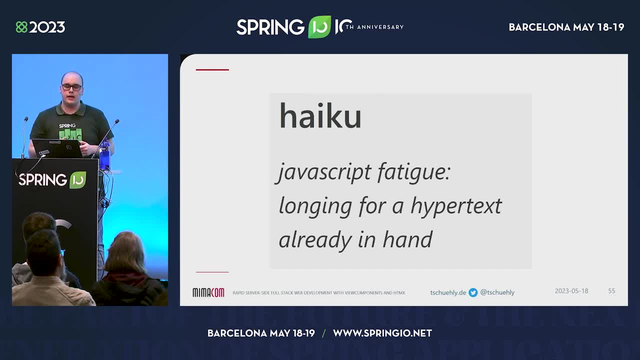 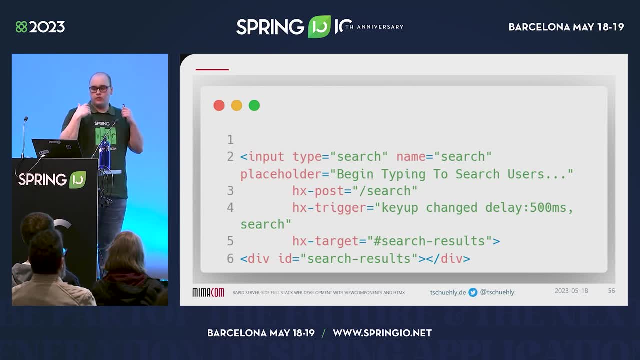 state with the superior user experience of a single-page application. HTMX enables us to enable UX patterns that are only commonly known with single-page applications, like active search. This input triggers a single-page application. Here is a post request to the search endpoint on key up that is debounced by 500 milliseconds. 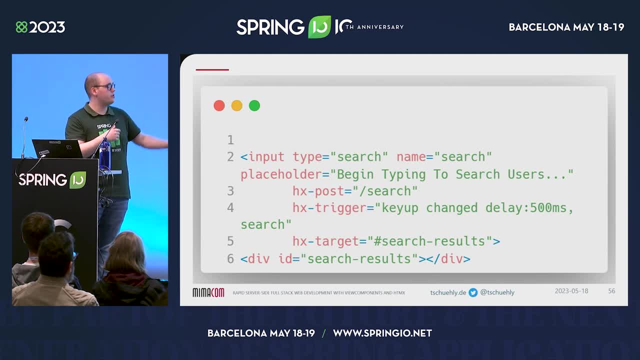 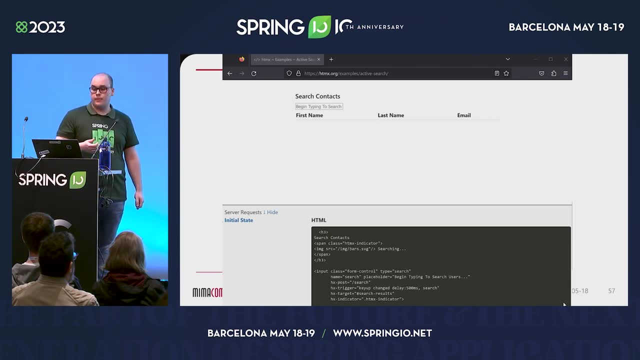 Then the response is swapped into the search results element. Here is an active search example on htmxorg. It has the same experience as a single-page application, without any of the complexity. You can see the essential characteristics of a hypermedia-driven application, Our front-end. 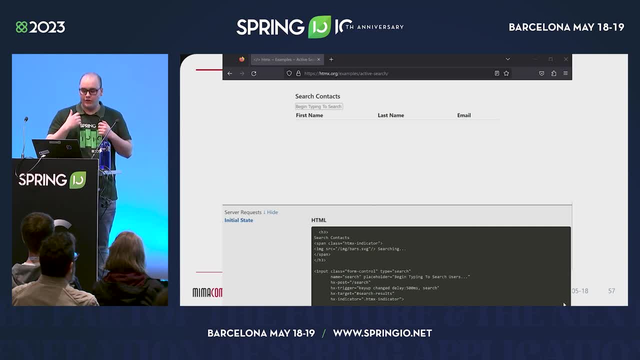 is entirely declarative. We have a single-page application without any of the complexity. You can see the essential characteristics of a single-page application without any of the complexity. Our front-end is entirely specified in declarative HTMX attributes right inside our HTML. 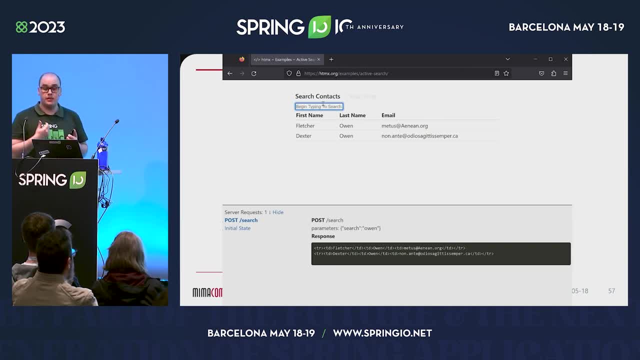 As you can see, the interaction is done entirely over HTTP and HTML. HTMX makes requests for us and swaps the HTML that gets returned into the DOM. It is not a far-fetched idea to think that if HTML would have had one of these attributes, we would have been able to do the same thing. 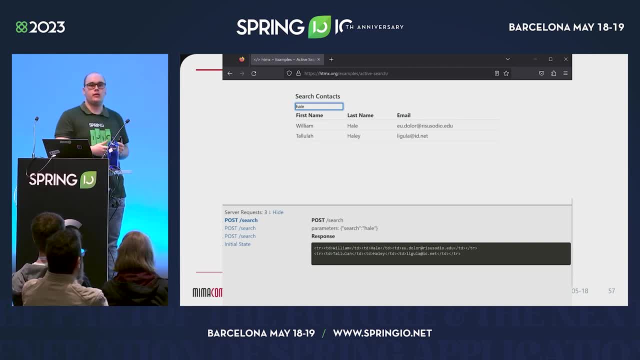 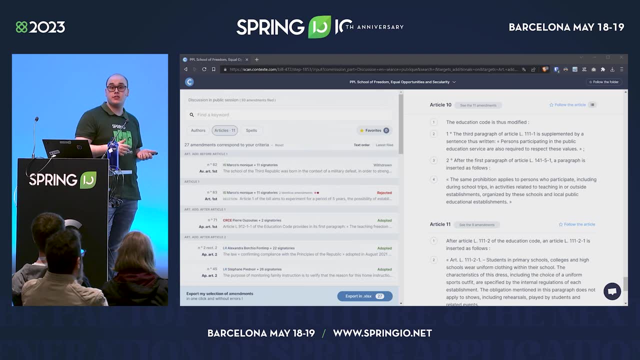 in HTML. The fact is that we are all in this together. We have been involved further as a hypermedia. This could be native HTML enabled by our browser. As with everything, there are advantages and disadvantages we need to consider when engineering our software. 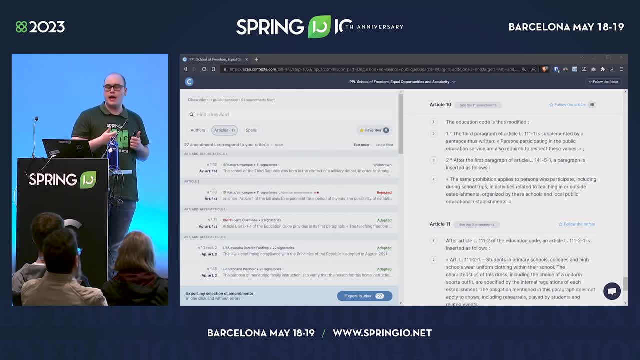 Hypermedia-driven applications are especially good if your UI is mostly text and images, for example, a news article site that serves media to our users. Here is a real world example of HTMX. It's a software as a service startup context. They track legislation in the French Senate and show amendments. 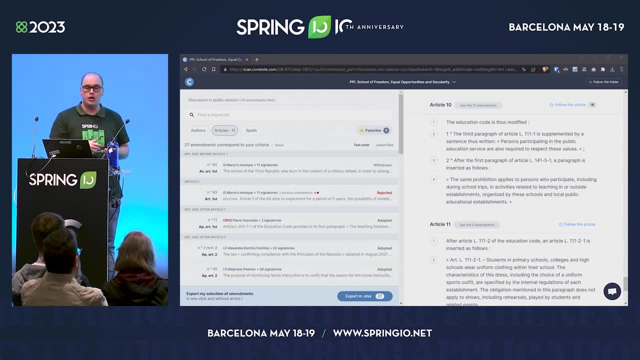 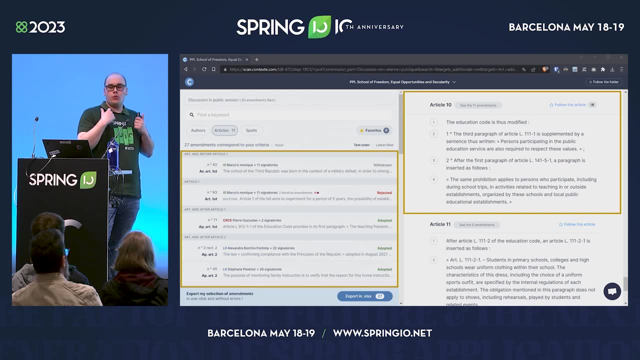 They transition successfully from a Django plus React application to a Django plus HTMX application. If your UI is nested and the blocks are well defined, it is easy to create dynamic interaction. This lends itself especially to the view component approach, as we can just re-render our components. 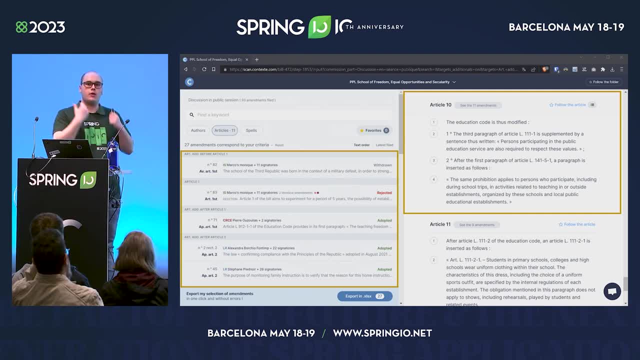 on demand, We get out-of-the-box first-page render performance. that is perfect in search engine optimisation, as it is just standard HTML. As I've alluded to earlier, there are use cases where a JavaScript-centric approach makes more sense if we need a high degree of sub-millisecond interactivity, for example. 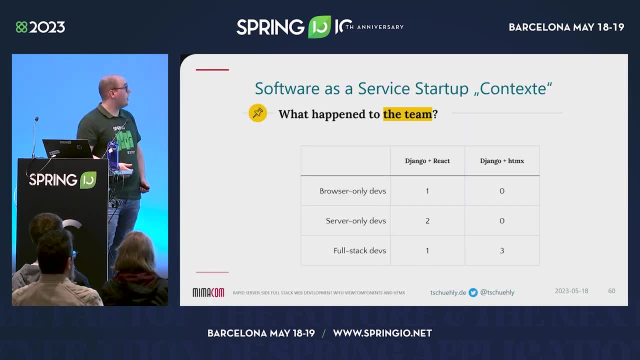 Google Sheets. Now I've talked. We've talked about why and how we can create a hypermedia-driven application, but what should not be overlooked is how the team structure can change if we radically simplify our web development approach. When Context was using React, they had a hard split between back-end and front-end developers. 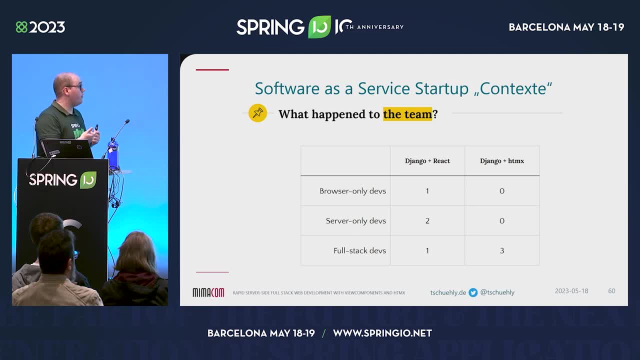 Two developers were entirely back-end, one developer was entirely front-end and one was full-stack. After the port, the entire team became full-stack developers, except the JavaScript developers. He didn't have a job anymore. Each team member is more effective and able to contribute more value. 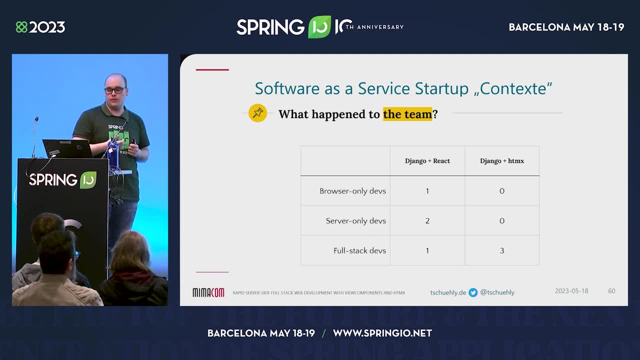 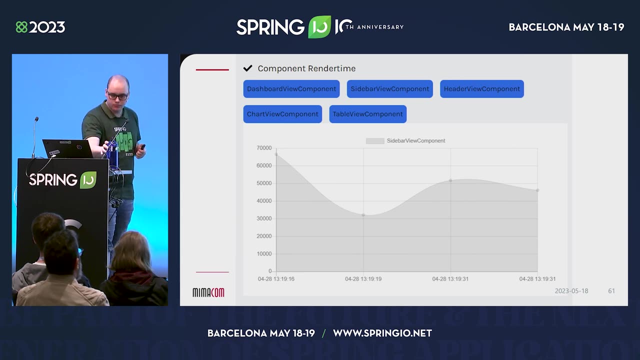 The development is more fun as they can own an entire feature. It leads to better optimised software, as they can make optimisations anywhere across the stack without any co-ordination. Spring View Component nicely integrates with HTML. This example: I created an analytics service that measures the render time of each view. 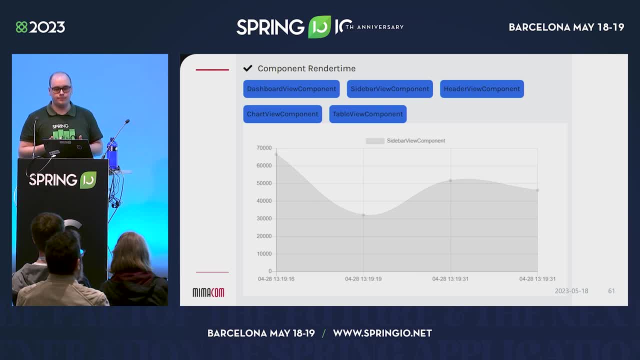 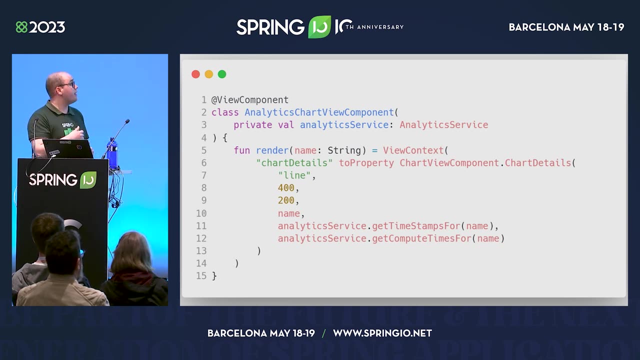 component using the aspect-oriented programming support of Spring. We want to show a chart for each component to our user. Obviously, we don't want any reloads. for a nice user experience, I've created the Analytics Chart View component that auto-wires the analytics service. 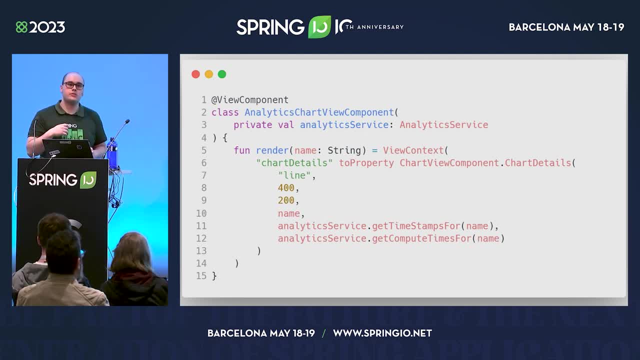 We then create a chart with the generic Chart View component that wraps the Chartjs library in a type-safe envelope. As you can see, the View component self-describes the API through the ChartDetails class. We can see what chart it is. We can specify the width and the height, the name, the data and the labels for the data. 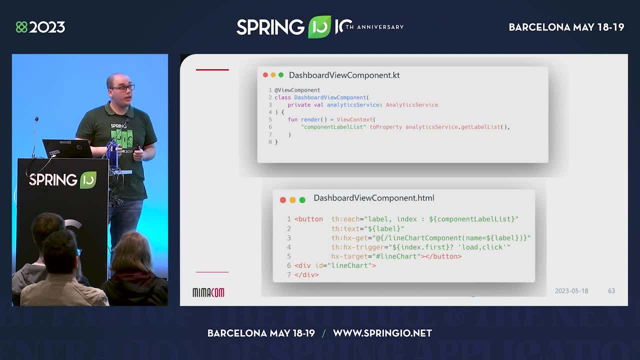 Next we look at the Dashboard View component. We get all components by name from our analytics service as component label lists and then reference each component by name In our HTML. at the bottom you can see that we loop over this list with a th-each attribute. 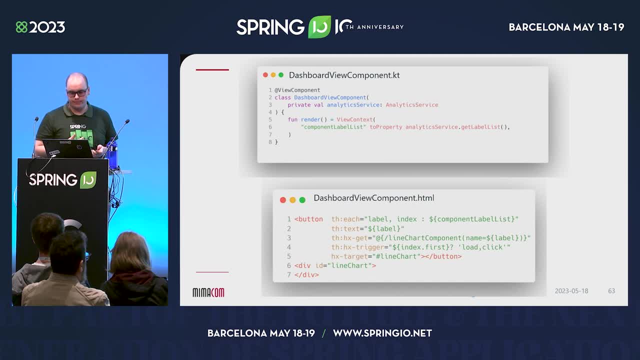 We set the button text with the th-text attribute. Then with the th-hx-get attribute we can create GET requests to our slash line chart component endpoint. We pass the request parameter name with the reference name. Of course, this is a nice way to think about the data bar to our Atlas and we can easily 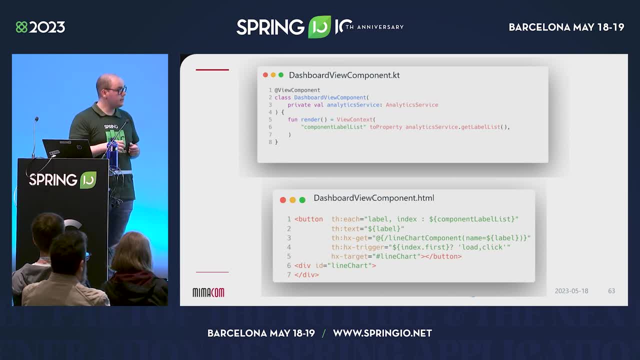 fix what the data bar is doing: variable name. This creates get request. to this end point, To need to know what HTML should be swapped, we add the hx target attribute with the slash, with the line chart ID. We then add an hx trigger attribute and add it only for the first element, that the first. 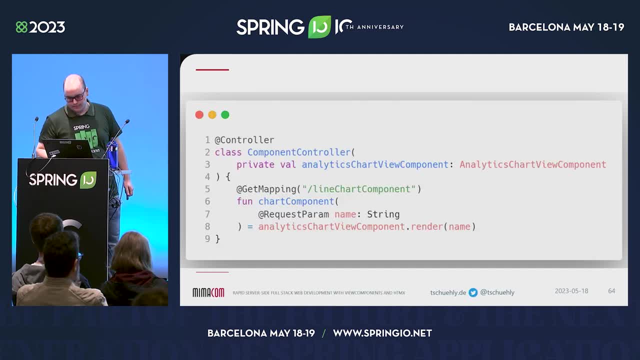 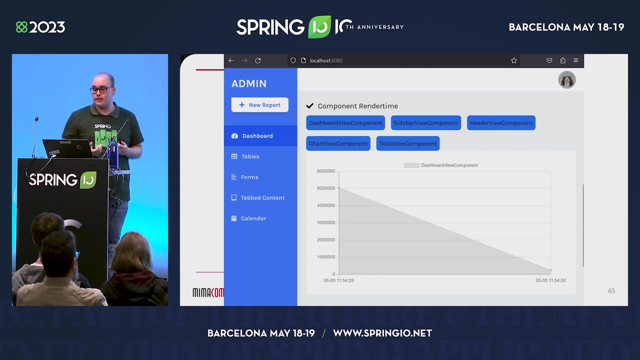 element loads on page load. We then create a component controller. This auto-vias the analytics chart view component as it is just a spring bean. Then we create a get mapping slash line chart component and add a request parameter name. Then we return the analytics chart view component with the name as parameter. This is the example implemented. 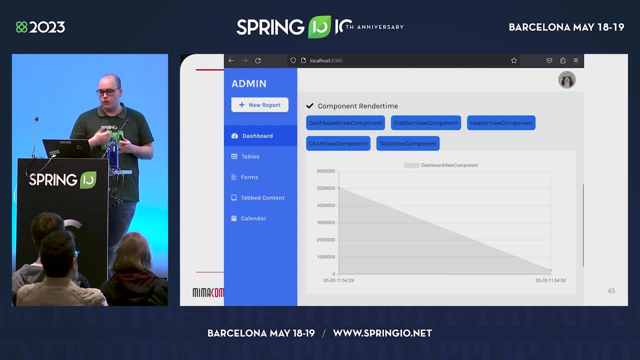 to show you the fully interactive application without any page refreshes. As you can see, the user can just click on a button and the data updates automatically. It also works across page reloads, so you can see that there are new data points after. 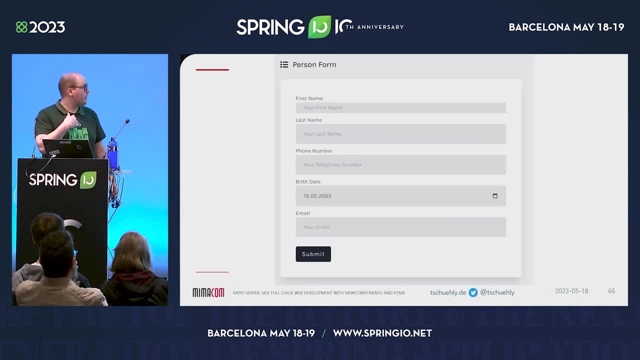 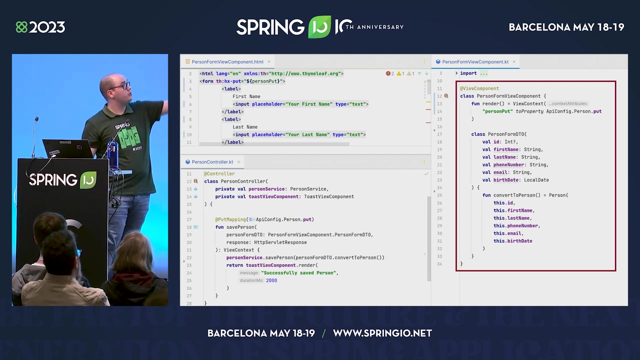 reloading. Next I will show you how we can create, how we can leverage the component to create highly cohesive and loosely coupled features. We want to enable our user to save a person to a database. On the right you can see the person component. We create the person put variable with our 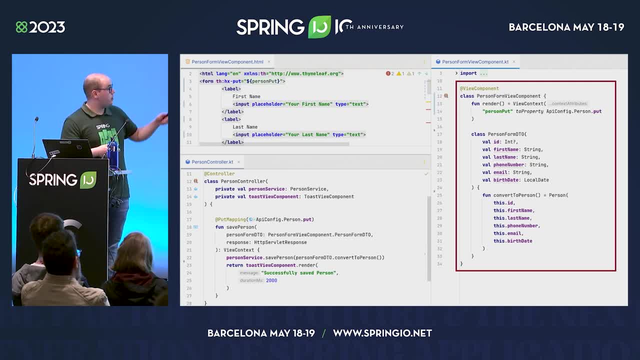 API config. Then below you can see the person form DTO. This describes the HTML form you can see. Then below you can see the person form DTO. This describes the HTML form you can see. on the topic left The form is defined. then we add an HX put attribute where we put the person put. 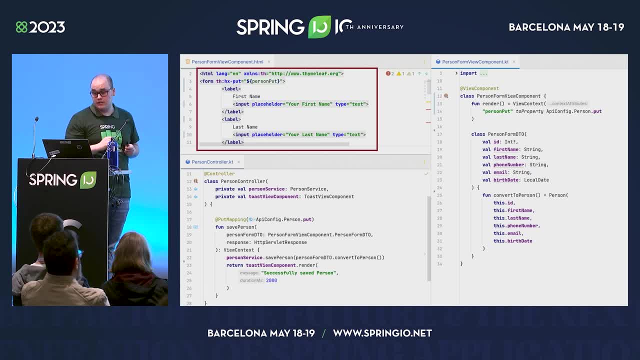 as variable. Then below you can see the input fields that match the DTO class in our view component. On the bottom left you can see the person controller that is responsible for saving the person when submitting the form. We reuse our API config with the person. 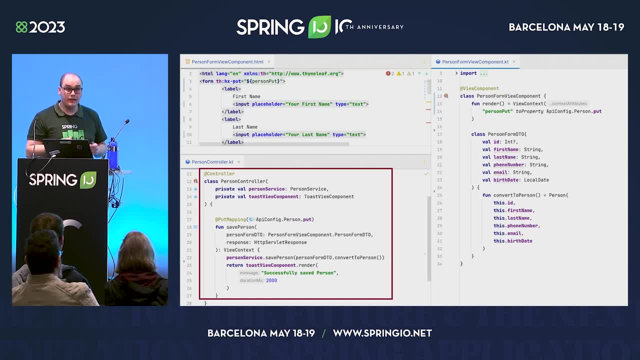 put in our put mapping. We don't care if the path changes, as it still works. The person form view DTO is our method parameter. so if we change the form and the DTO, the controller doesn't care because it doesn't own the class. When we save the person with the person service, 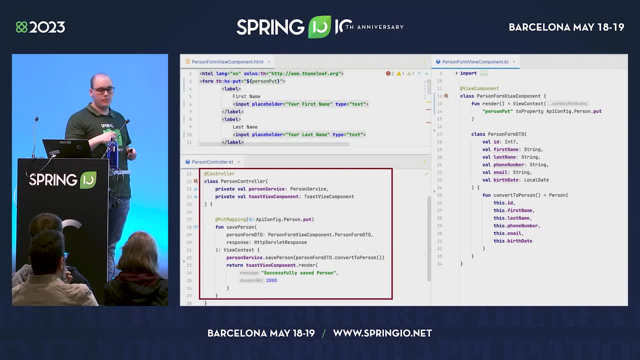 we use the person form DTO, dot convert person method. so when we convert the person DTO to our person domain object, the dependency only points inward, enabling us to create features in a clean architecture style. Then we return the toast view component dot render method. It shows a message to our users that he saved the person. 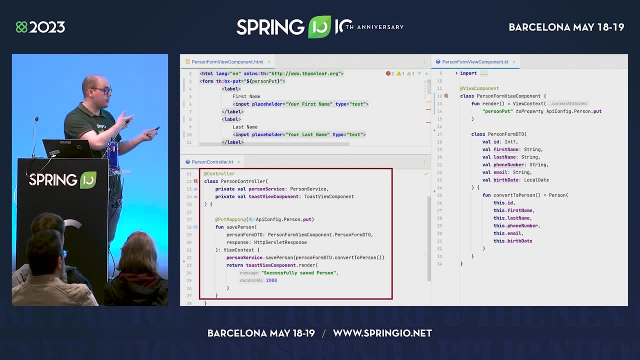 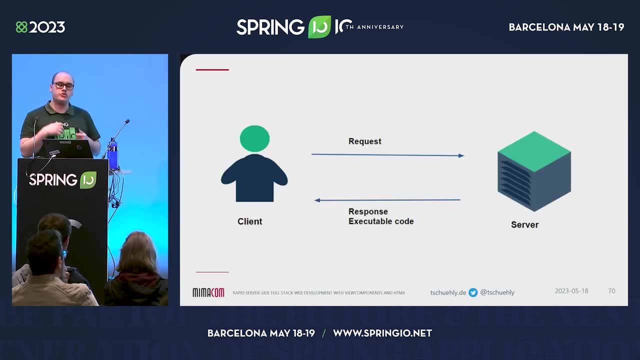 The message successfully saved persons for two seconds. That's another good example for a reusable view component. We can further improve the interactivity of our hypermedia-driven applications with the optional constraint, called on demand, of the rest architecture style. We embed JavaScript right inside our components to enable client-side interaction. 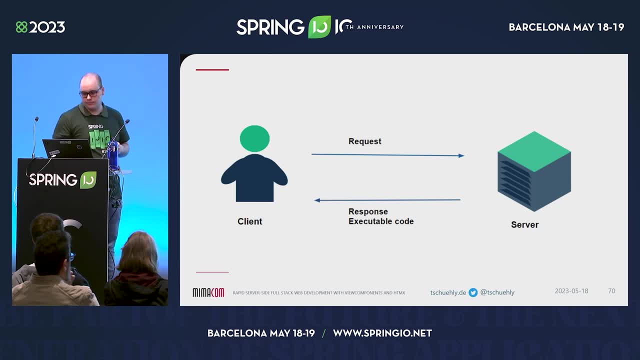 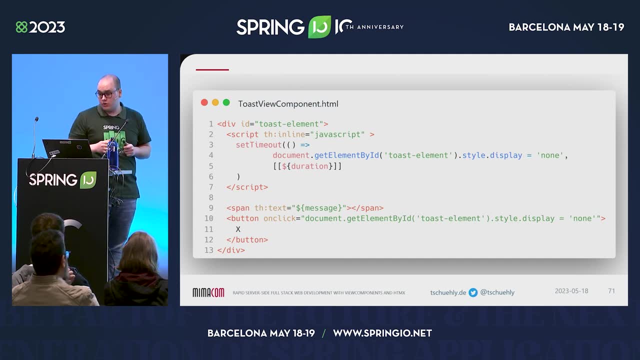 but we satisfy the locality of behaviour design principle. This is the HTML of the toast view component we used earlier. We embedded JavaScript with a little script tag that gets auto executed when we return the HTML snippet from our server. In this example we used a. 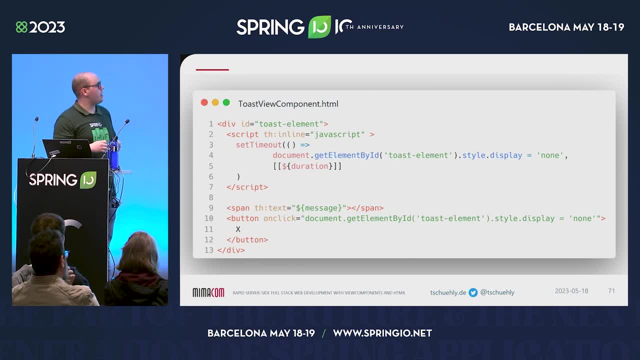 set timeout. function that sets the style dot display element style dot display attribute to none after the duration. we pass to the method We show the message with the TH text attribute and we enable our users with the on click to faster hide the message. We can. 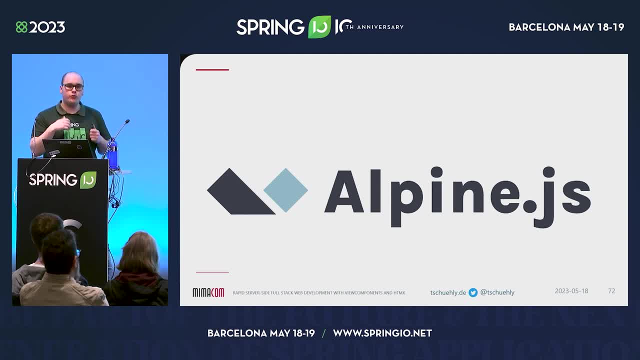 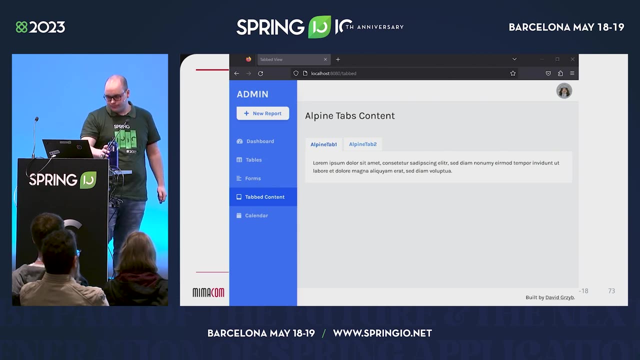 use JavaScript for client-side interactivity, but I've really liked the approach of the Alpine JS library. It is a minimal tool to create interactive front-end behaviour inside our HTML with 14 attributes. Here is a sample view component that shows the power of Alpine JS in combination with: 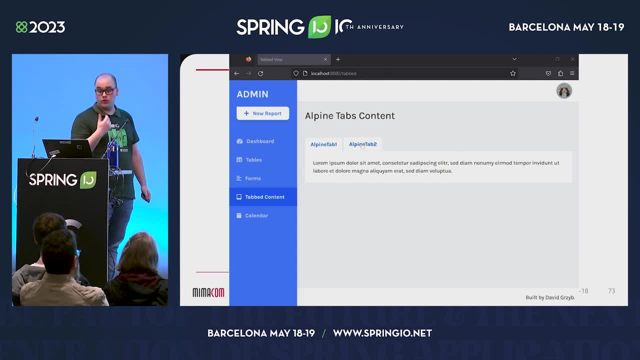 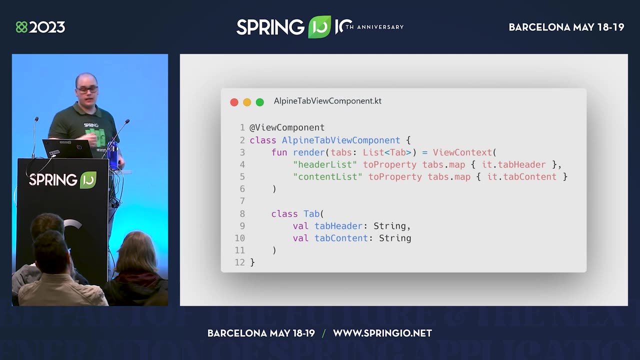 view components. It is a reusable tab view component we can reuse anywhere across our app for switching content client-side. This is the AlpineTabViewComponentkt. We can see that we have a list of tabs as parameter that maps them in our view context. 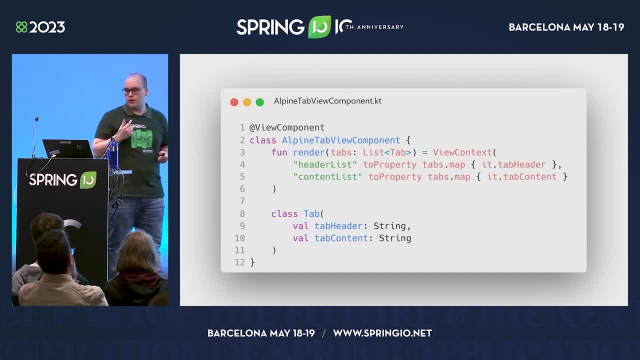 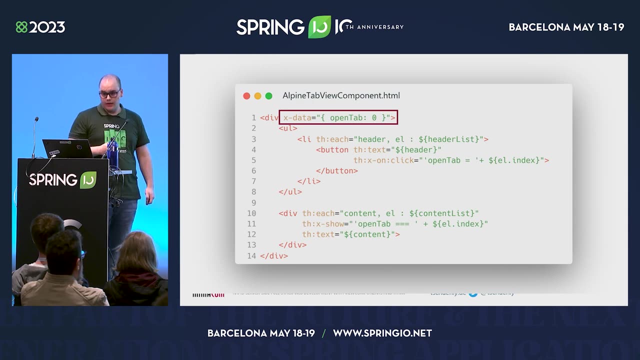 We list these tabs to two lists: the header list and the content list. It shows the power of view components, as we can define the API of the component in our class type: save. The AlpineTabViewComponenthtml template consists of the AlpineJS xdata attribute. 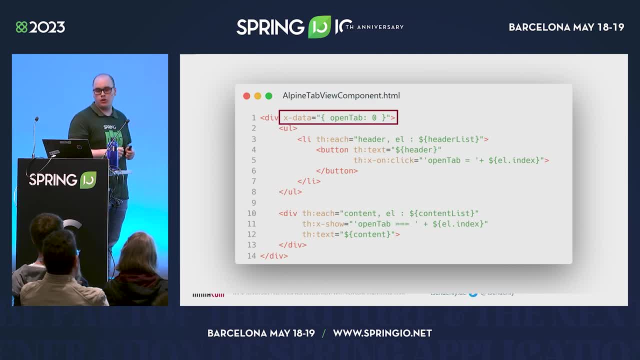 We define a variable scope and we set the OpenTab variable with the value set to zero in the scope. With the timely th each attribute we can repeat the list elements for each item in our header list, for example here. Then With the button element we show the text of the header variable we created in our th. 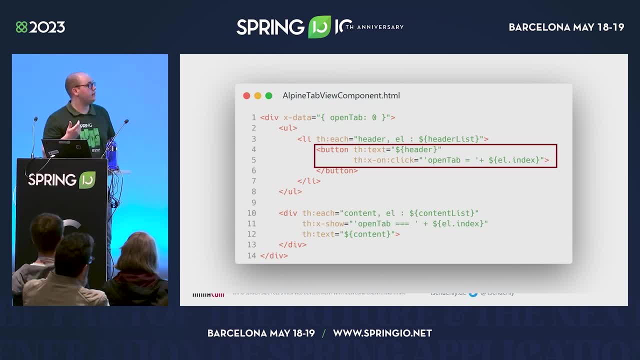 each. and then we use the th xon click to set the OpenTab to the index of the element in our list. When the user clicks on a button, the OpenTab variable is set to the index of the element. Finally, we show the content in our div. 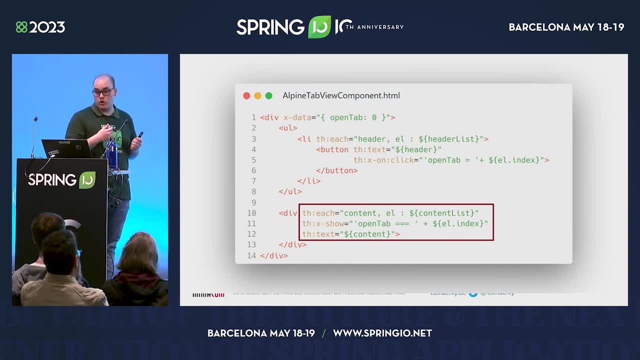 For each item in our content list. With the AlpineXShow attribute we toggle the visibility of our header element with the header element with the same index We set. with the th text attribute we set the inner HTML of our content from our content. 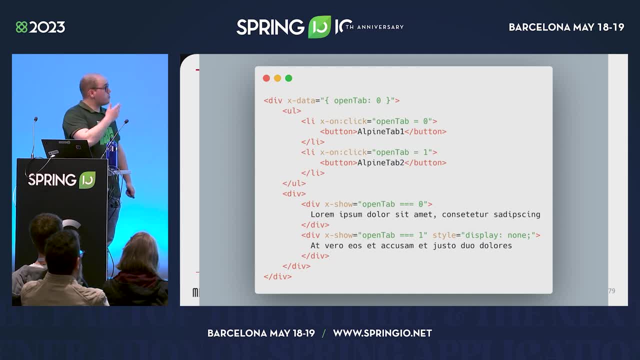 list. This example is the rendered HTML that shows the power of combining Thymleaf with AlpineJS. You can see that Thymleaf created two list elements, each with an XonClick attribute that sets the OpenTap variable to the respective index in our scope. 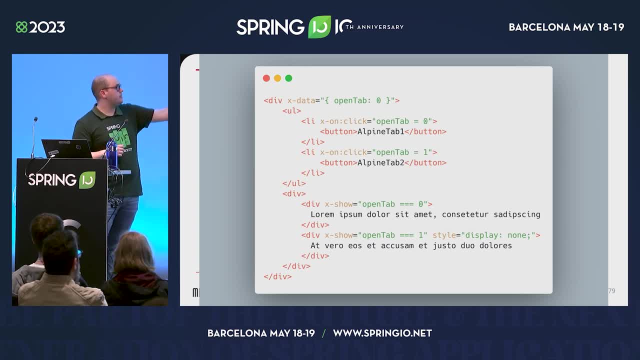 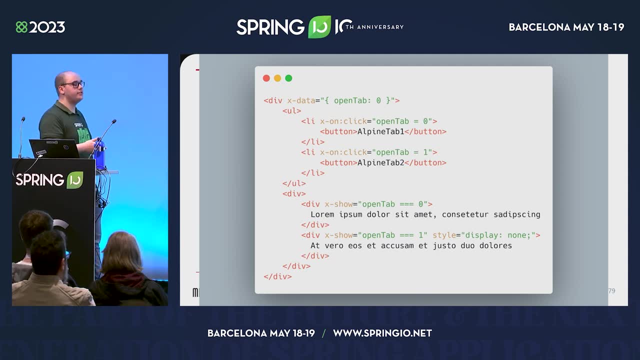 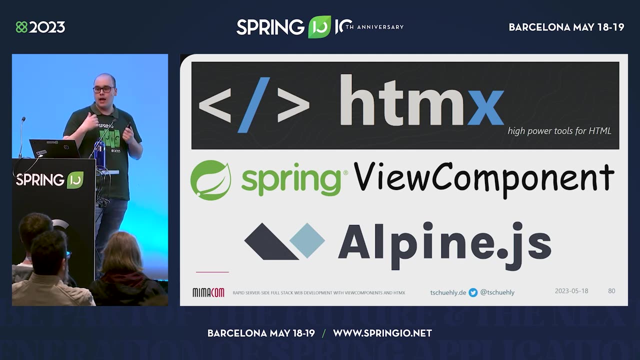 Then you can see in the content area that on the OpenTap equals zero, there's a style display- none added, so it doesn't show as the OpenTap variable is zero and not one. Now I showed you how to create interactive hypermedia-based web applications with SpringView components, HGMAX and AlpineJS. 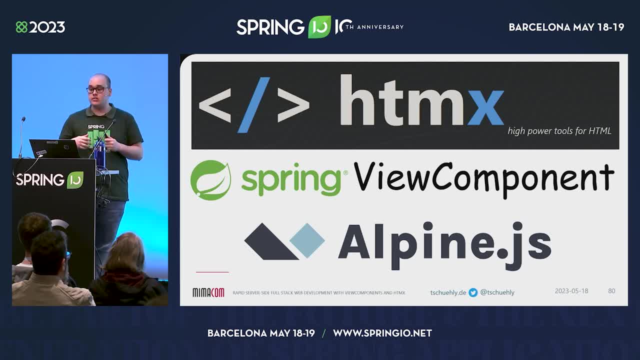 But to further close the gap in terms of productivity, we need to address the integrations all these JavaScript frameworks provide, because they have a definite edge for smaller projects and indie hackers. as they provide integrations, for example, for authentication, They get from zero to production much faster than we can. 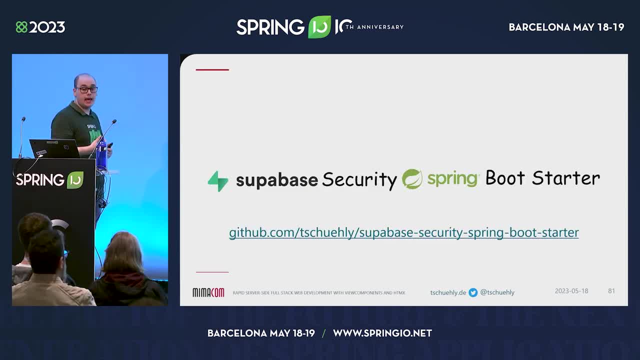 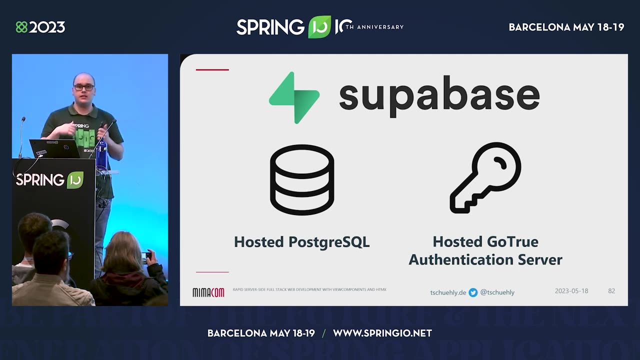 To close the gap I created the SuperBase Security SpringBoot Starter. It enables authentication and database hosting really easily with SuperBase. SuperBase is an open-source Firebase alternative that has two features that are especially interesting for our full-stack web apps. The first is that SuperBase offers a hosted Postgres database that we can connect like any JDBC database. 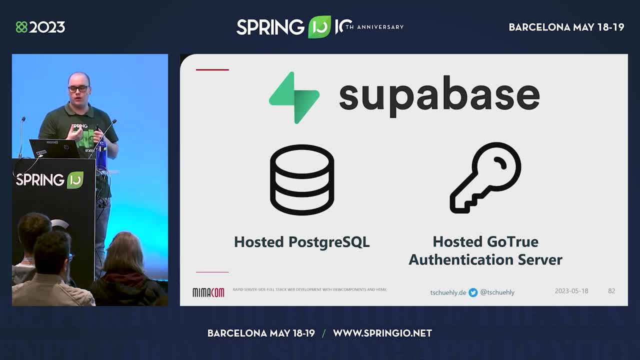 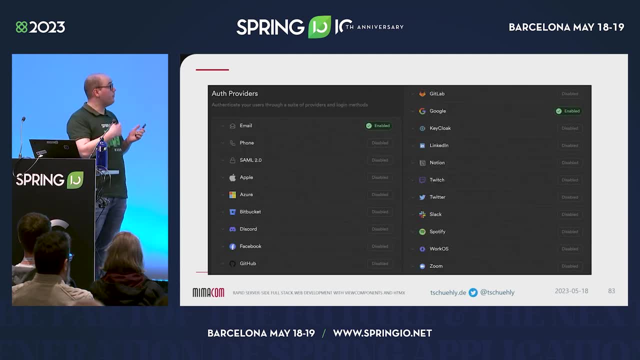 SuperBase offers a hosted Postgres database that we can connect like any JDBC database. SuperBase also offers us a hosted GoToServer so we can move the responsibility of storing user credentials to SuperBase. We can configure email authentication and other authentications really easily in the SuperBase dashboards. 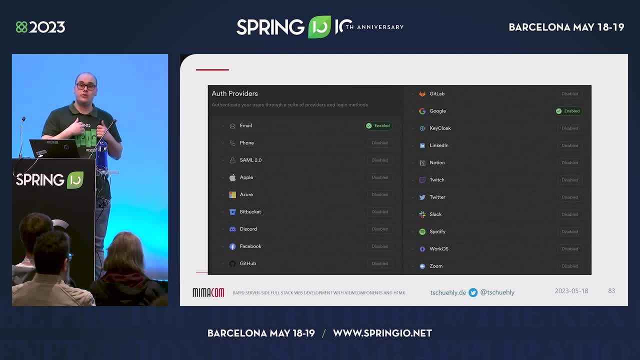 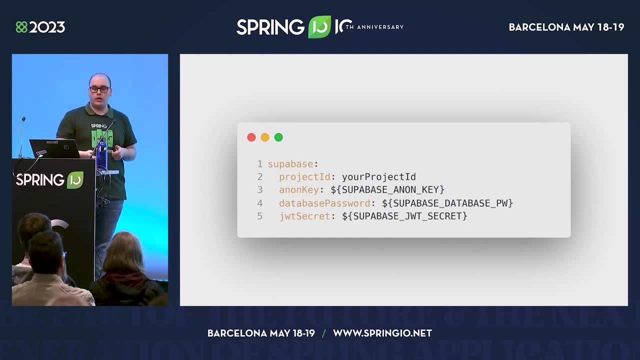 SuperBase handles verification and password-forget emails, so we don't need to build that ourselves. After we include the SuperBase starter, we can configure the project ID that SuperBase gives us. Then we need to define the NN key, the database password and the JWTC grid so we can mint our own JWTs. 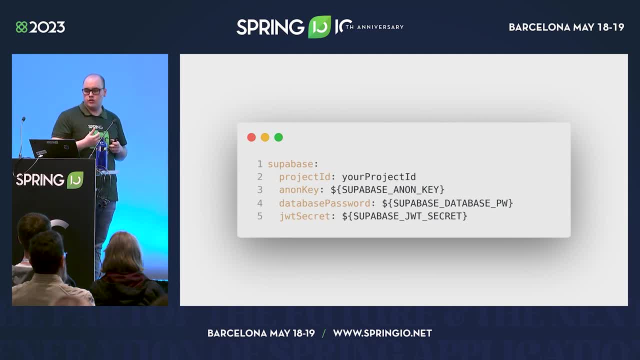 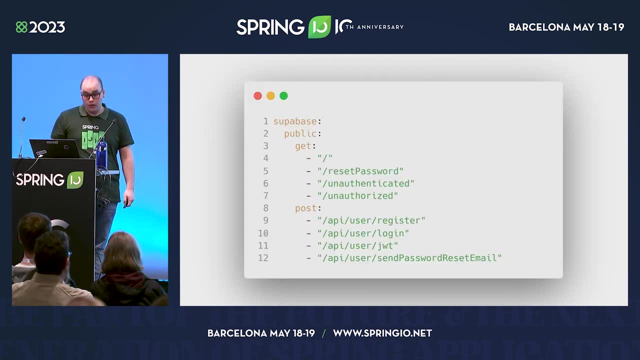 This will also set up the JDBC data connections automatically and set SuperBase as SpringBoot security provider. We then can configure our security right inside our applicationyaml. Here we include some endpoints that the SuperBase starter automatically creates, But we can register any endpoint in our YAML for any HTTP method. 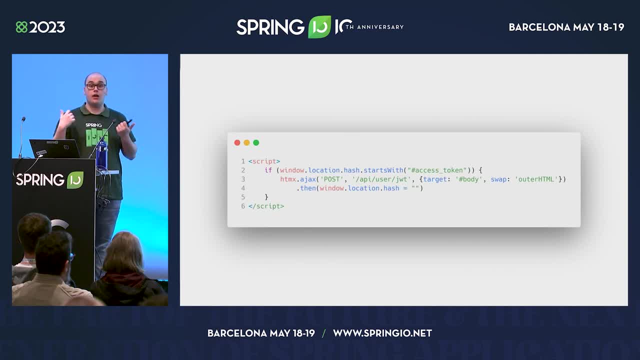 The starter is heavily optimized for HTMX, but it can also be used for JSON. API SuperBase uses JWT as an authentication method. So after an email confirmation or after an OAuth login, we get a JWT in our URI fragment. We leverage the htmxajax method to send the JWT to our apiuserjwt endpoint. 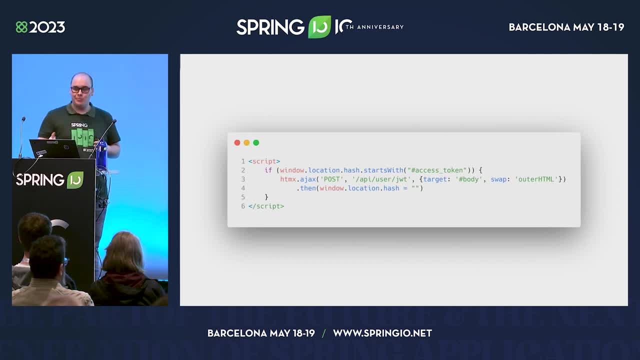 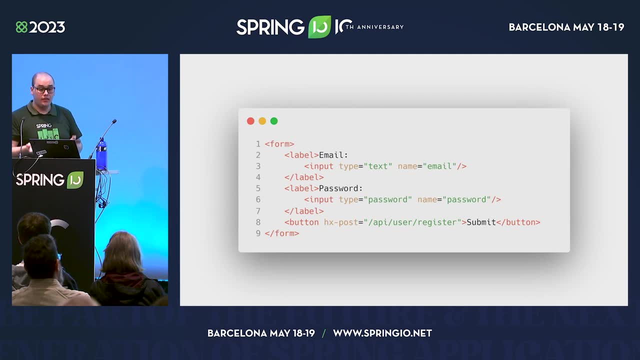 which then saves it into a cookie that persists it across page reloads and navigations. After setting everything up, the email registration form is easy. It's just an ajax post attribute to our apiuserregister endpoint that is submitted with HTMX. The same is true for the user login. 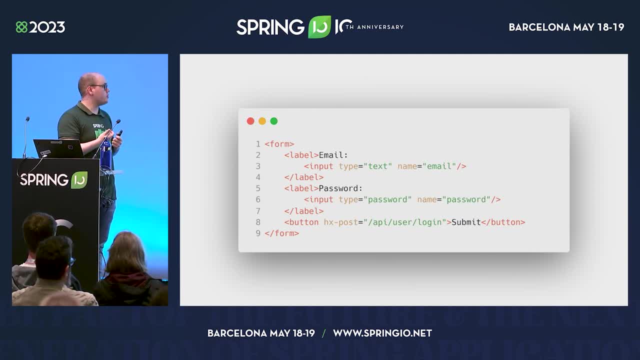 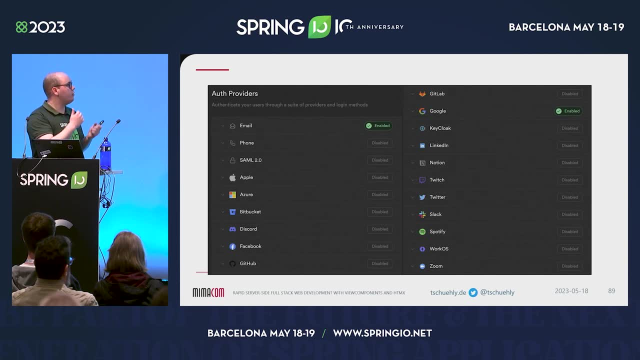 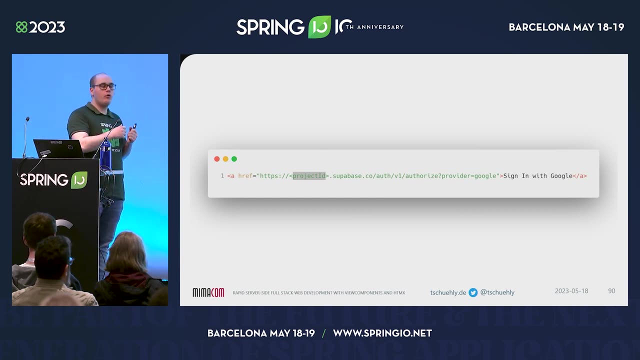 That's all that's needed for setting up authentication- Just two forms. We can also enable other OAuth providers- like here we did with Google in the SuperBase dashboard- To create the Google login. we just use a link that redirects to the Google login. 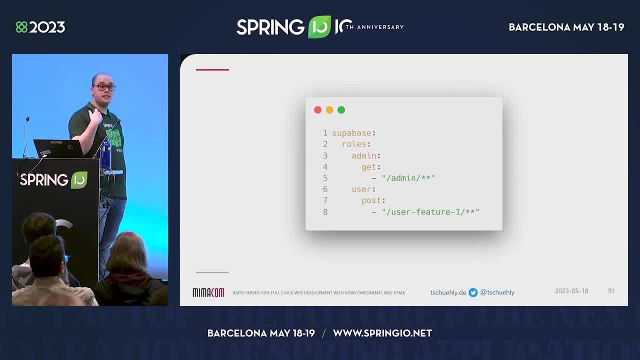 With SuperBase security we can also create role-based accounts. We can also create role-based authorization for any role in our role array. in our applicationyaml We can fine-tune it for any HTTP method that this role has access to. With this config, you can see that the admin role has access to the admin endpoint with the HTTP method get. 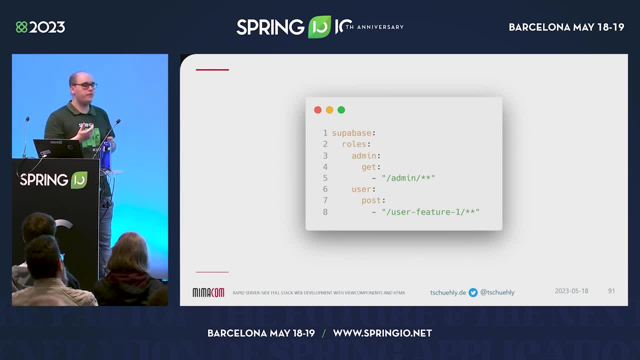 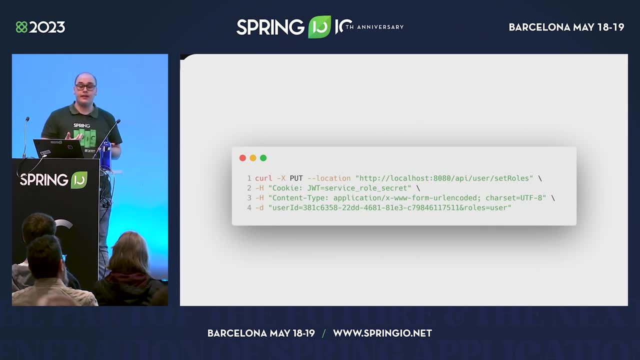 And the user role has access to the user feature endpoints. with the HTTP method post, The starter exposes endpoints so we can set the roles of our users and create a role management system. We can use the endpoints with the service role secret we get in our SuperBase settings. 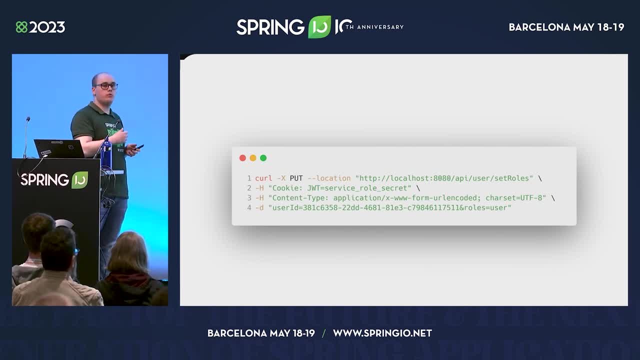 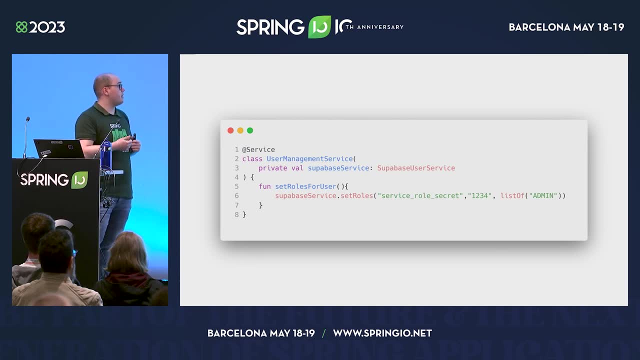 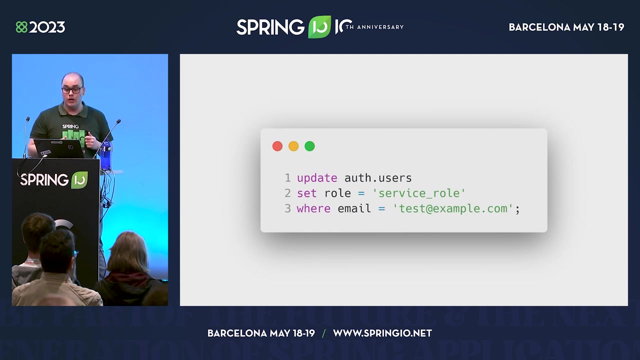 Here is an example: curl request. so we can set the role of this user to user. We can also auto-wire the SuperBase service directly. Here we set the roles of the user with the ID 1234 to admin. We can also elevate the privileges of a user with the service role secret if we set the role to service role. 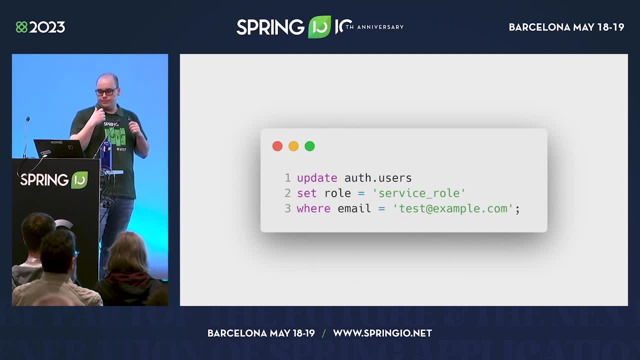 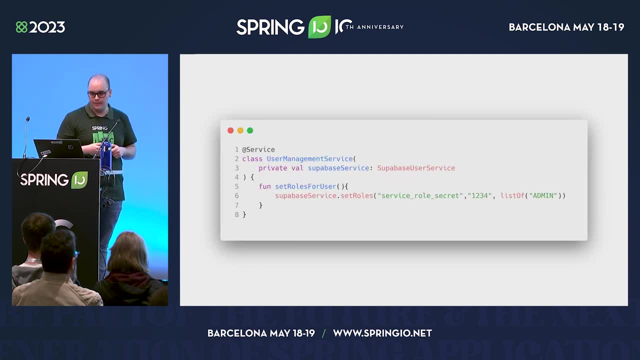 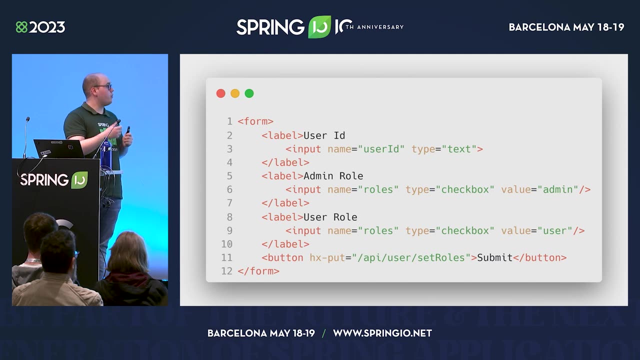 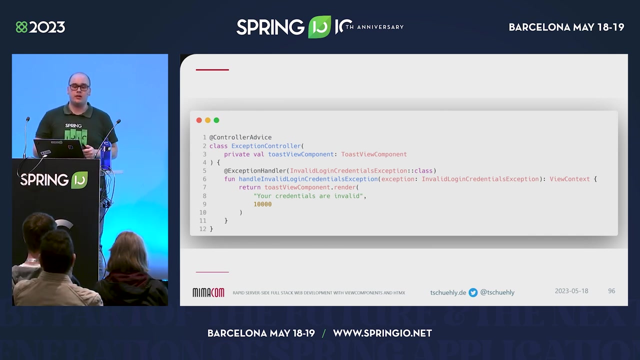 Then the user has the ability to set the roles of other users. We can use this form with the elevated user to set the roles of any users. It's that simple. The SuperBase security Spring Boot Starter exposes events through exceptions, So we can use a controller advice and an exception handler to pass messages to our user. 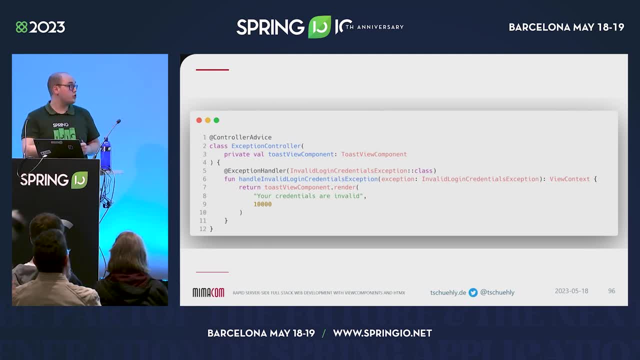 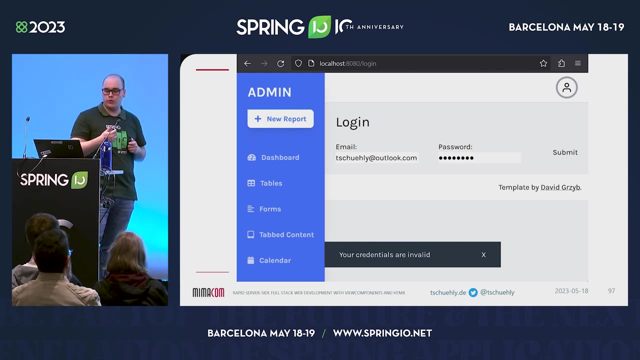 We leverage the SpringView components again As we want to show the user a toast that the credentials are invalid and show it for 10 seconds. Here you can see how it works. Here you can see how it looks when we try to log in with wrong credentials.